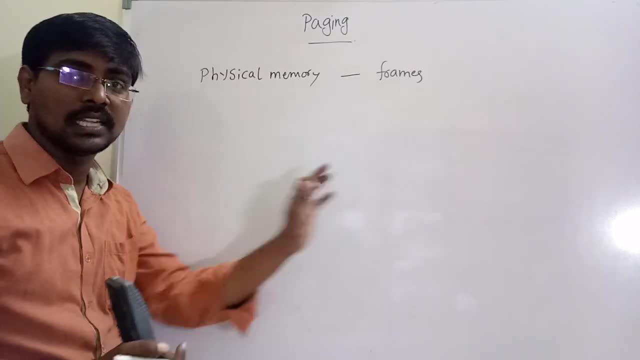 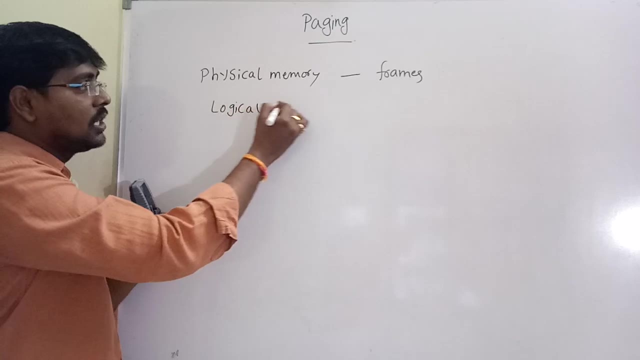 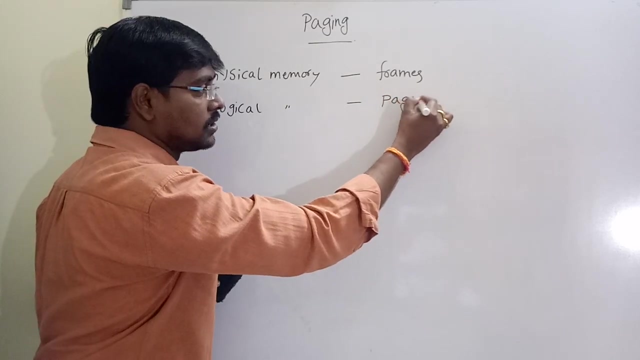 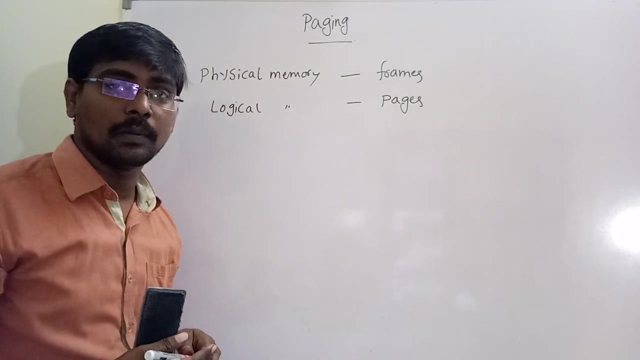 That is, the size of each frame is same. The size of each frame in the physical memory is same. Next, the logical memory is divided into fixed-sized blocks called pages. Fixed-sized blocks called pages. That is, the size of each page is same in the logical memory. 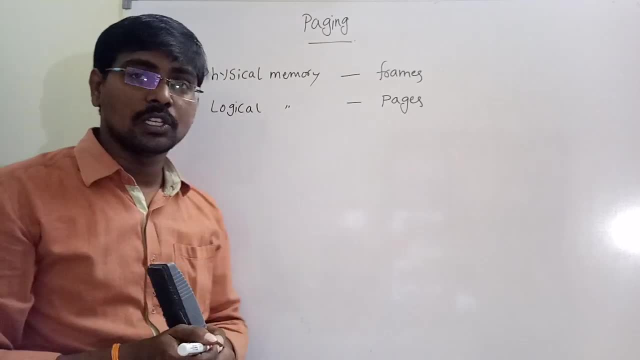 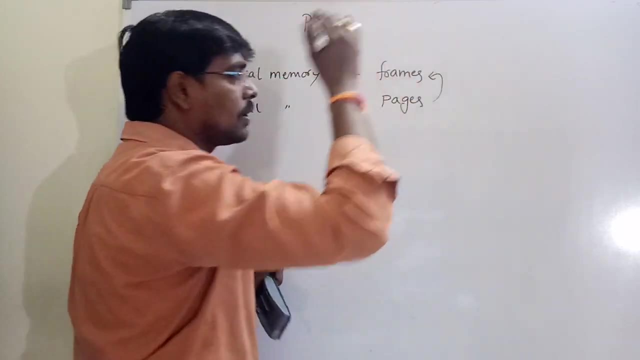 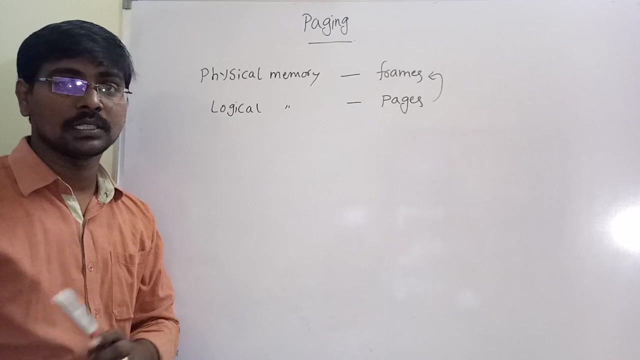 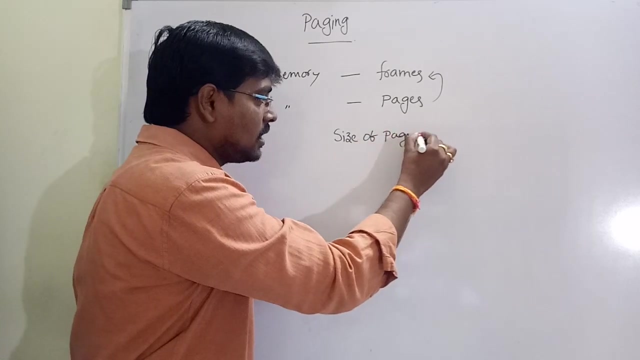 And whenever a process to be executed, the pages are to be loaded into the frames from the source Process to be executed, the pages are loaded into corresponding frame. That means the size of page. the size of page is equal to the size of frame. 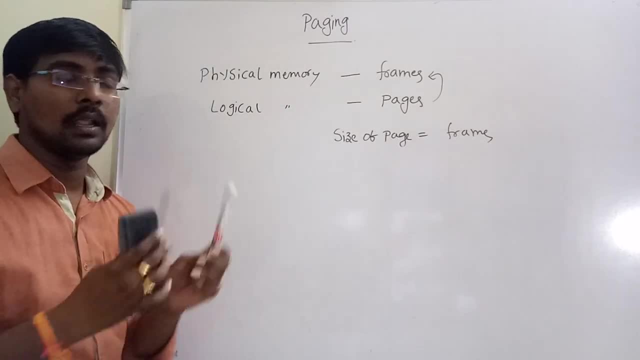 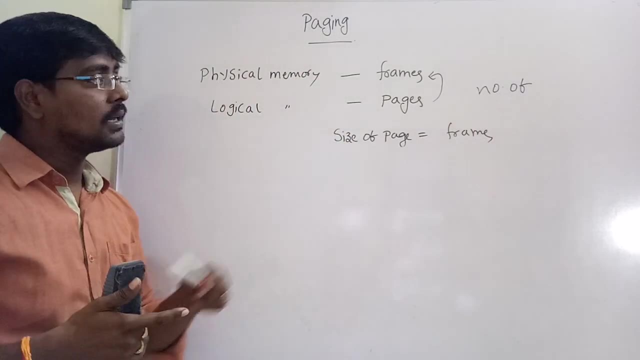 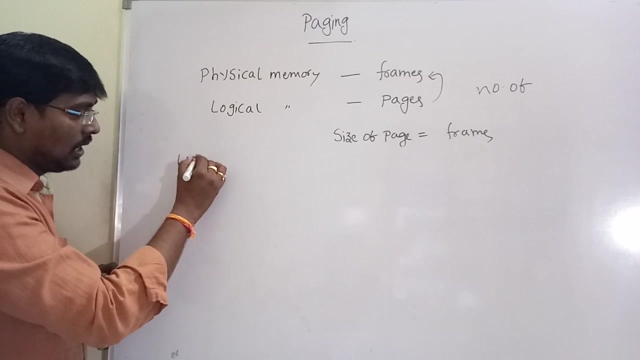 Page size and frame size must be equal, But the number difference, the number of pages and the number of frames may be different, But the size of page and the size of frames are same. Now see this one, The logical under space. 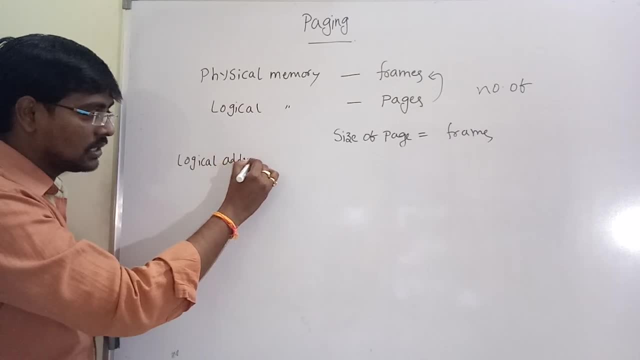 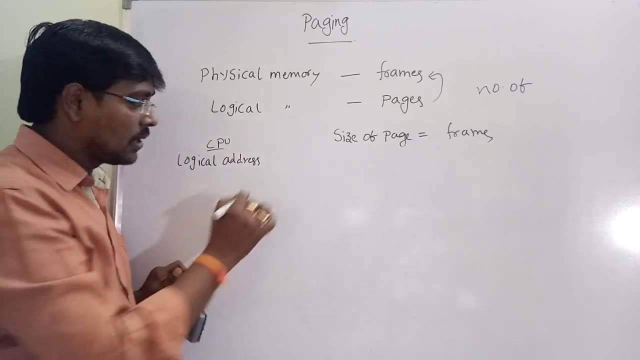 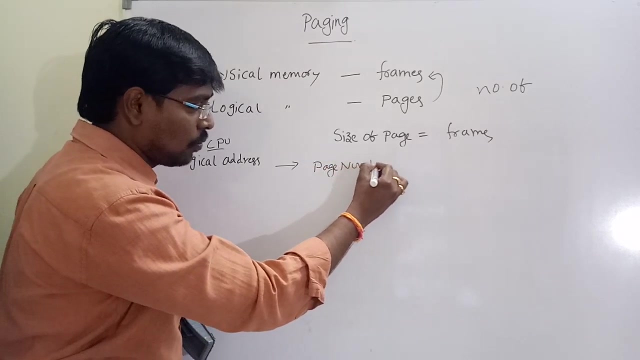 Okay, After division, the logical address. Who generates the logical address? The logical address is generated by the CPU. Address generated by the CPU is divided into two parts. One is page number. One is page number. Second, one is offset. Page number and offset. 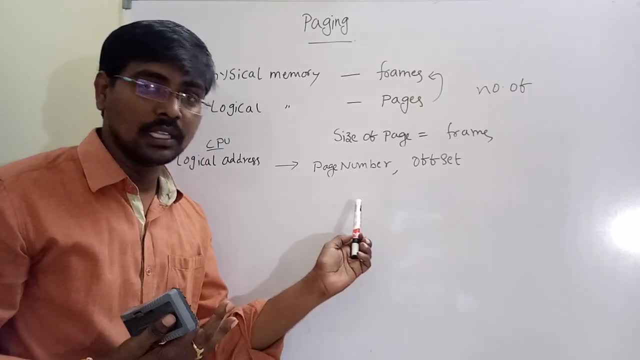 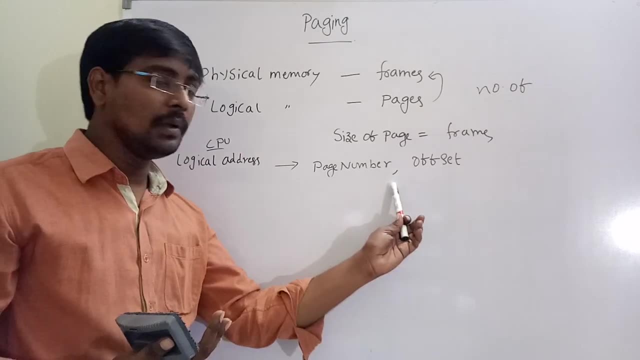 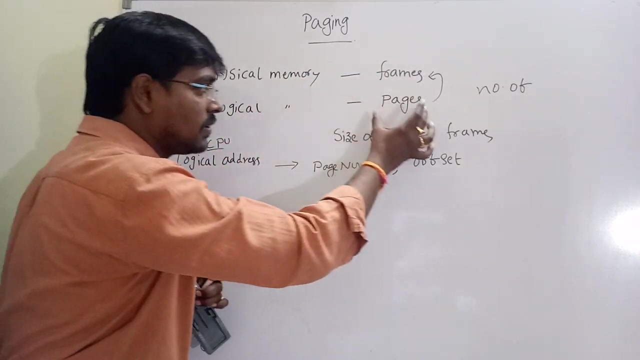 So by using page number, by using this page number, We are identifying the corresponding frame in the physical memory. How, In between, we have a page table. So see this one. The physical memory is divided into two frames. The logical memory is divided into two pages. 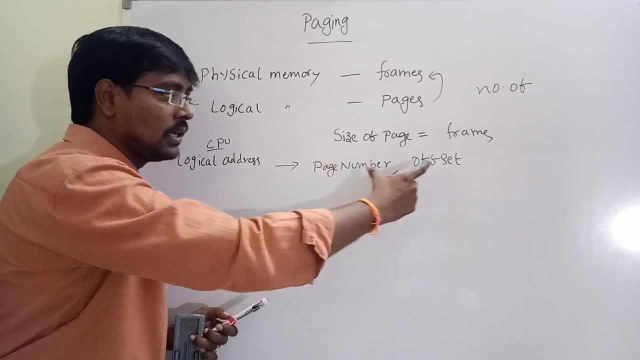 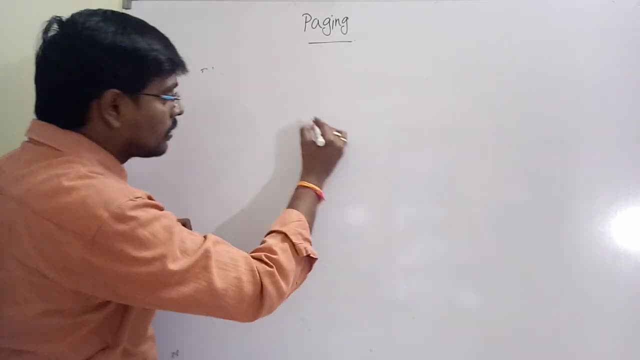 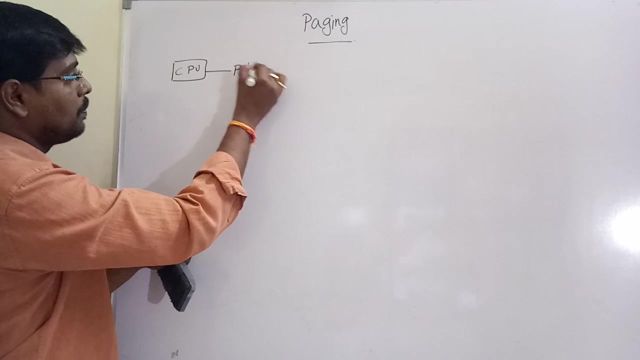 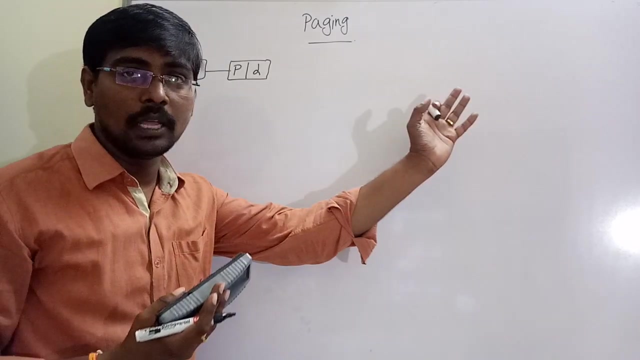 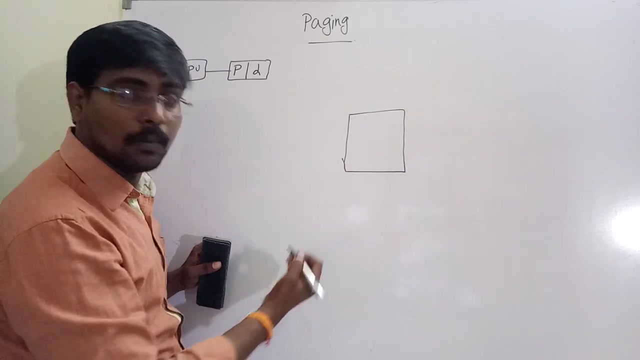 And the logical utter space is divided into two parts. One is the page number and another one is offset. Okay, Now move to the diagram. This is the CPU generated address. CPU generated address. CPU generates address is divided into P and D. Here P is the page number, D is offset. How we are mapping a two dimensional into one dimensional, similar to segmentation. Here we are using in the previous we are using segmentation table. Here we are using a page table. 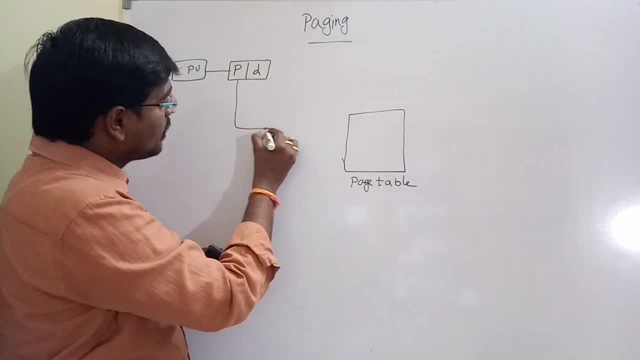 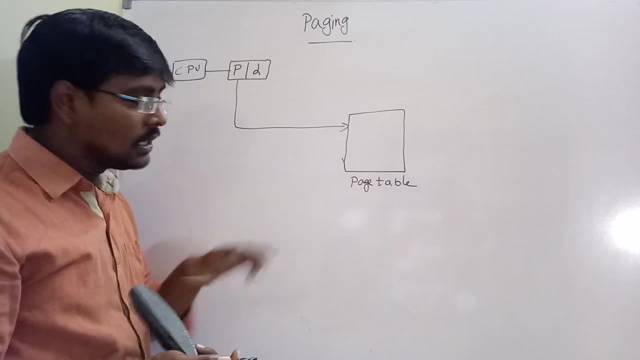 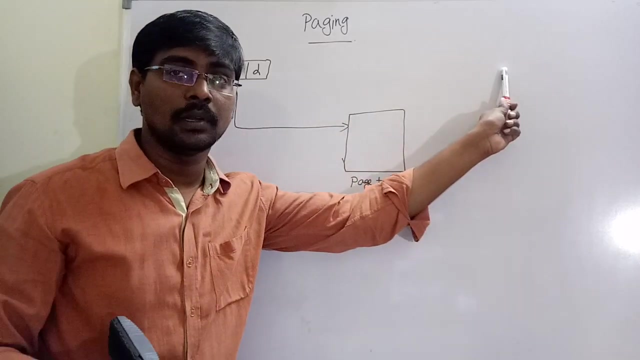 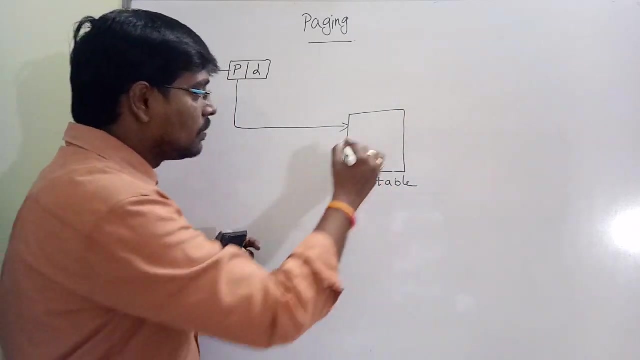 First, this page is checked, that is, the page number is checked in the page table. What the page table contains? Simply, the page table contains the base address of the page in the physical memory, That is, in which location, in which location this particular page is loaded. That is simply. it contains the frame number. 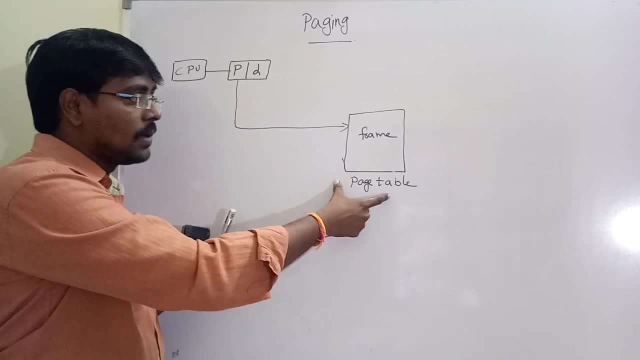 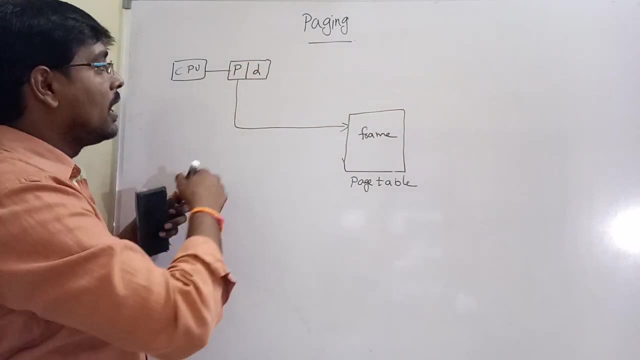 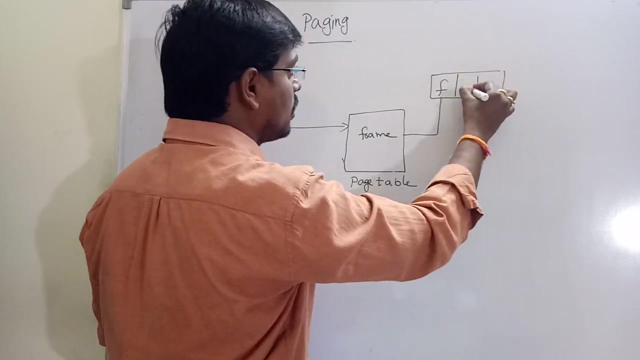 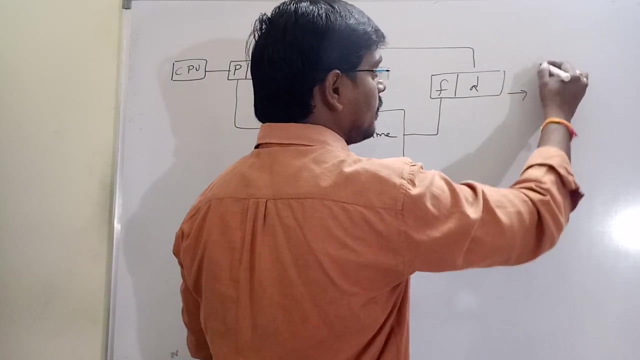 Ok, got the point. The page table contains the frame numbers at which address location, the base address of the page, And so this specifies frame number. This frame number is added to offset. The frame number is added to offset By adding simply: it is the location of physical memory. It is the location of physical memory. 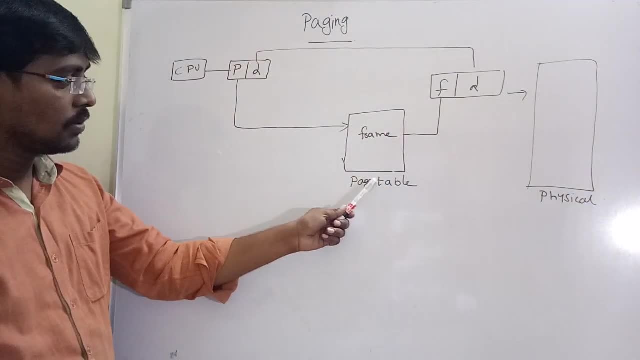 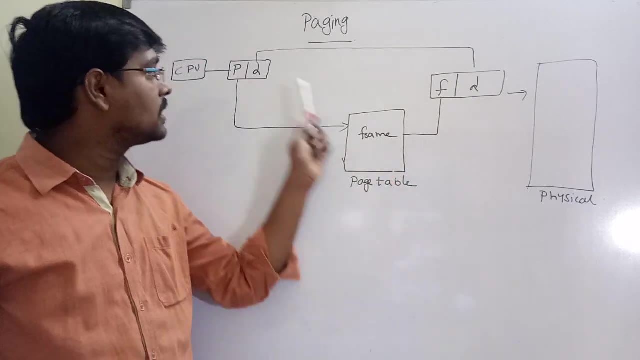 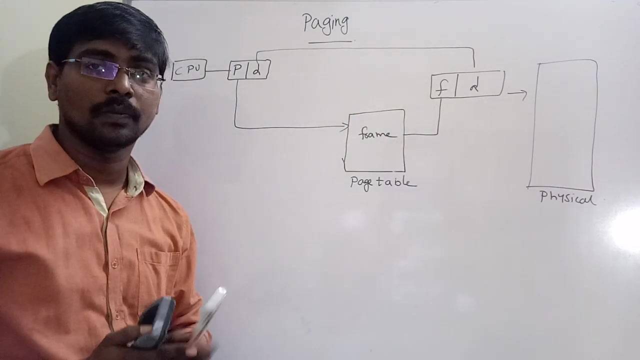 So you got the point, What the page table specifies. The page table specifies the base address of this page in the physical memory. For that base address I am adding offset Because the size of the page and the size of the frame are same. Page size and page frame are same. 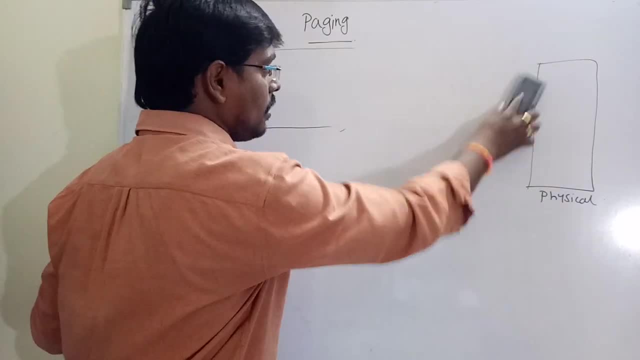 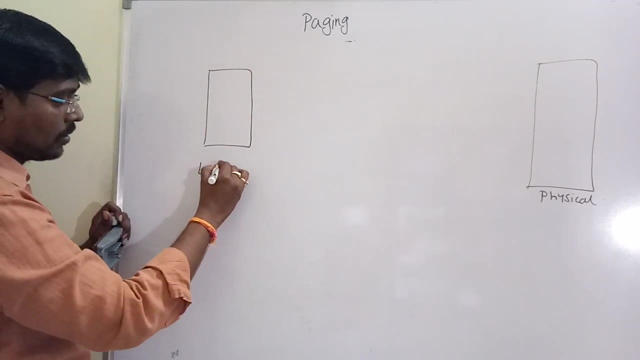 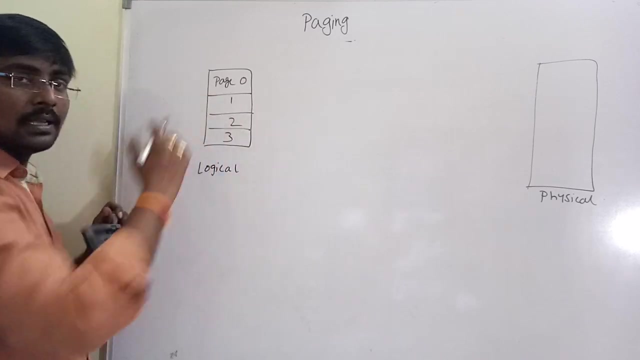 For example, assume this is the page table. Suppose we have logical memory Consists of some four pages: Page 0, page 1, page 2, page 3.. This is the logical memory Consists of four pages. 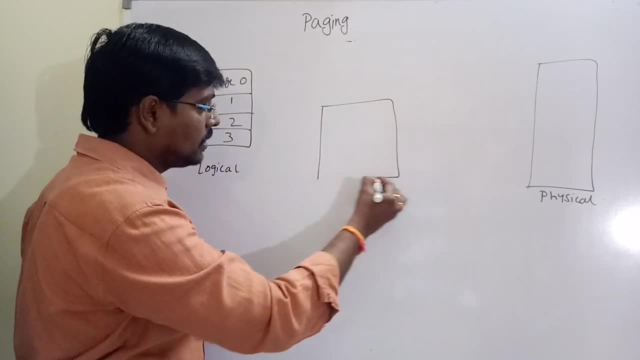 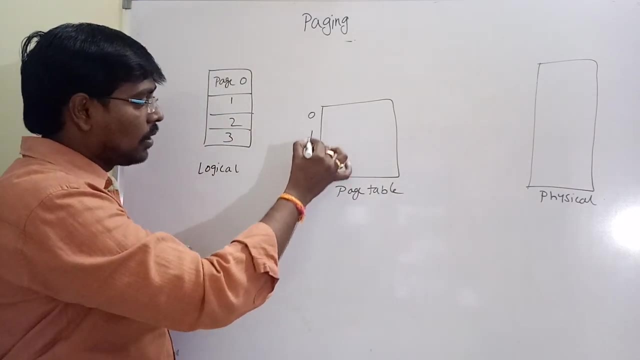 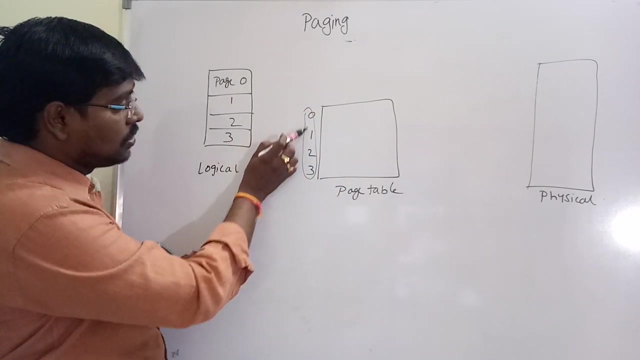 How the operation is performed means. This is the page table. This is the page table 0,, 1,, 2, 3.. What are these? These are page numbers. That is, page 0,, page 1, page 2,, page 3.. 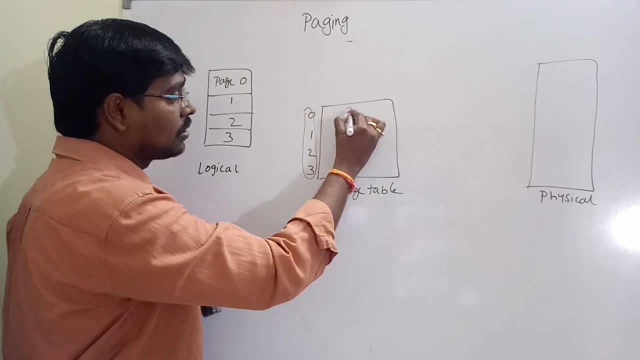 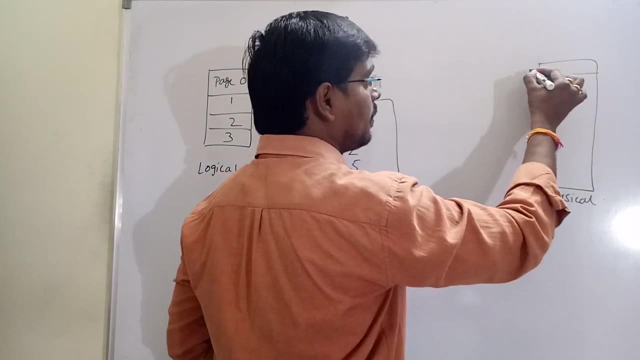 Suppose page 0,, 3,, 4,, 2, 5.. What is the meaning of, For example? this is the physical memory I am dividing to 0,, 1,, 2,, 3,, 4,, 5,, 6, 7.. 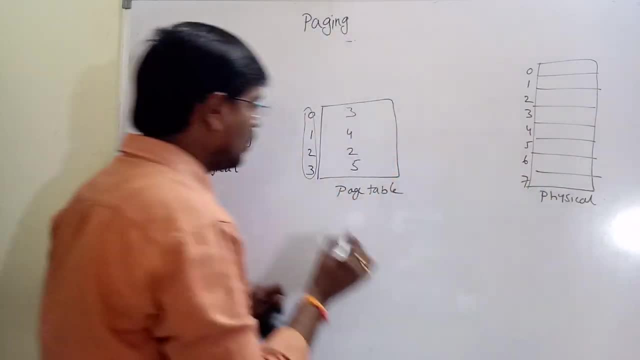 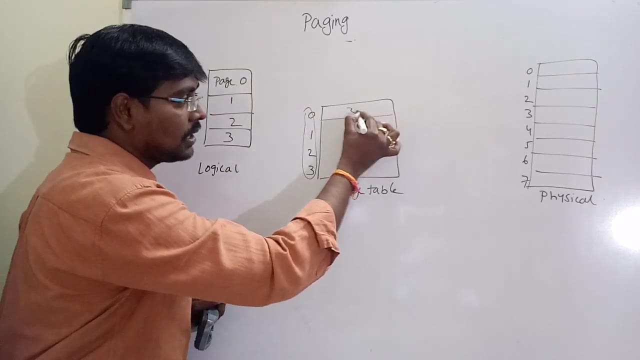 Suppose, if I divide in this fashion, How First page 0 is sectioned in the page table, What is the corresponding frame number? The frame number is 3.. Suppose this is the simple example. In this example, my offset is 0.. 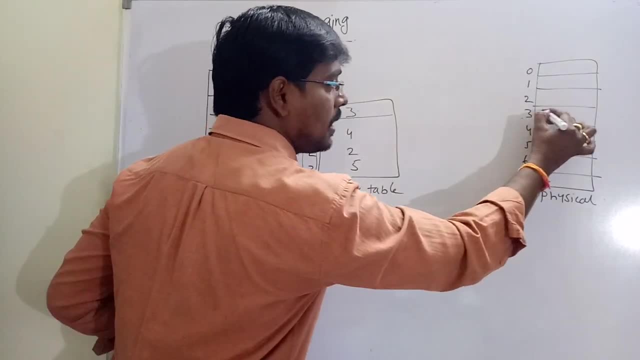 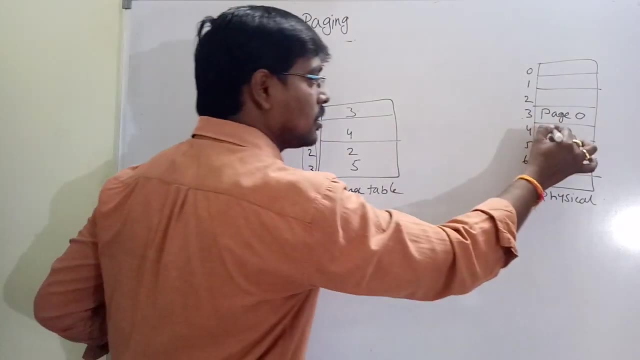 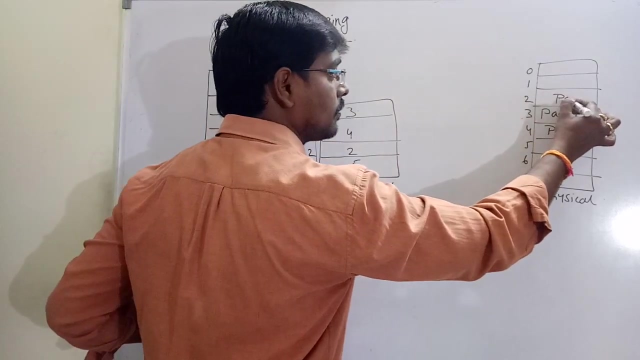 Suppose in frame 3.. That is this one. Page 0 is loaded Frame 3.. Page 0 is loaded Frame 4.. Page 1 is loaded Page Frame 2.. Page 2 is loaded In frame 5.. 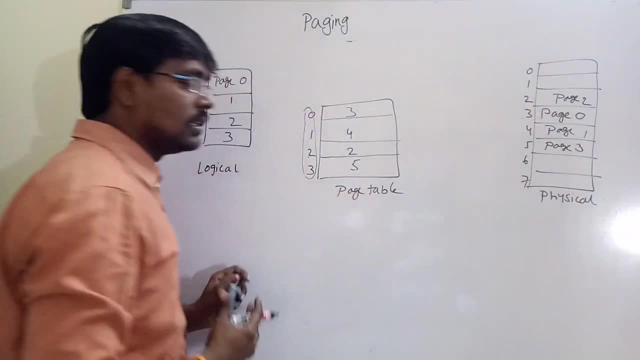 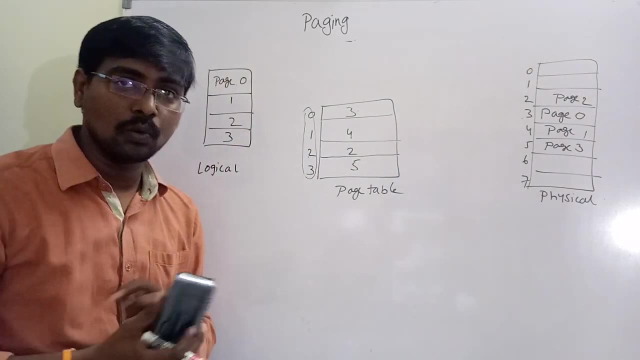 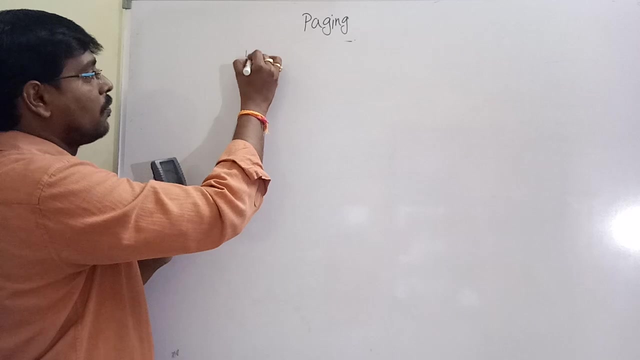 Page 3 is loaded. This is the way to map a page into the physical memory. This is all the pages with offset 0.. Now consider an example, Suppose. Consider an example In this example: 4 byte page. The size of page is 4 bytes. 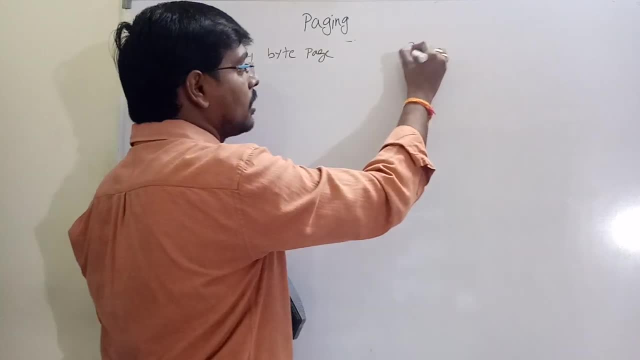 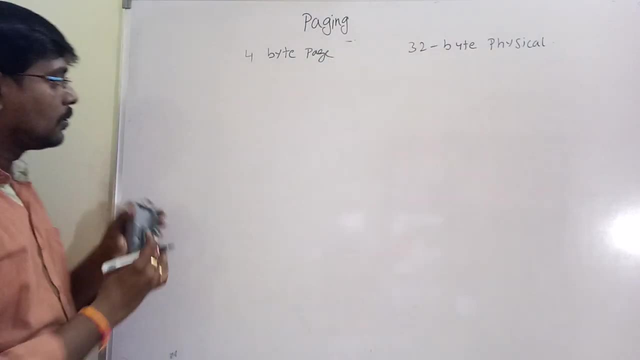 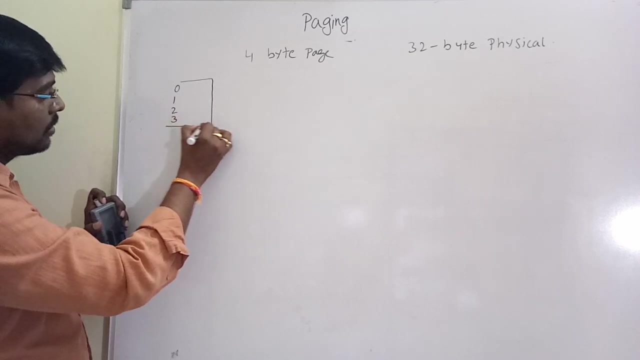 That is, each page contains 4 elements And 32 byte physical memory. 32 byte physical memory, Suppose- see the example- 0,, 1,, 2,, 3.. This is one page. This is one page, So size of page is: 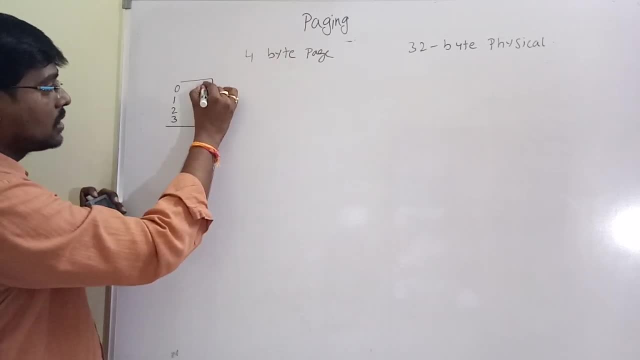 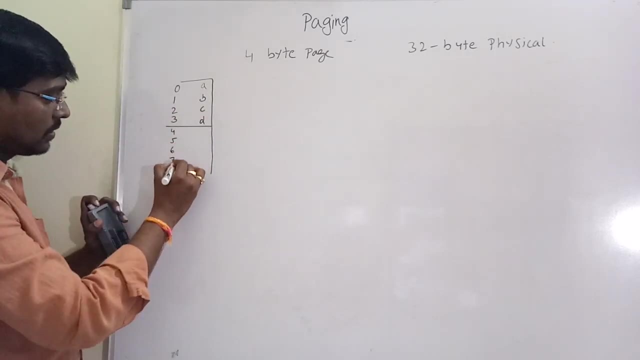 The size of the page is 4 bytes. Suppose A, B, C, D For our assumption. I am writing the names of the pages: 4,, 5,, 6,, 7.. 8,, 9,, 10,, 11.. 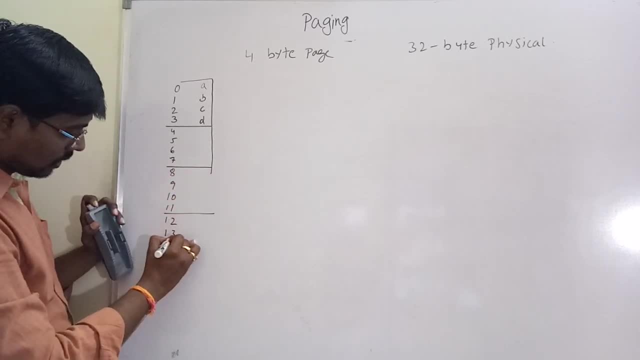 12, 13, 14, 15.. 12, 13, 14, 15.. 12, 13, 14, 15.. E F G H I J K. E F G H I J K. 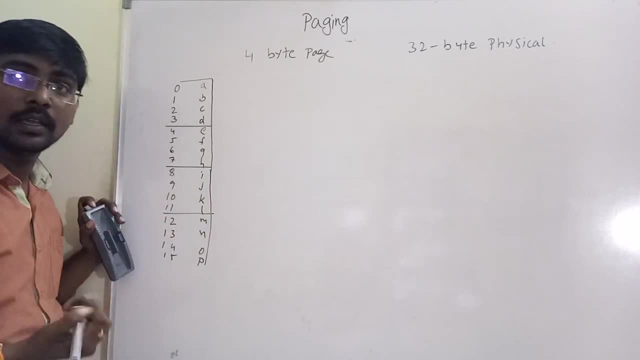 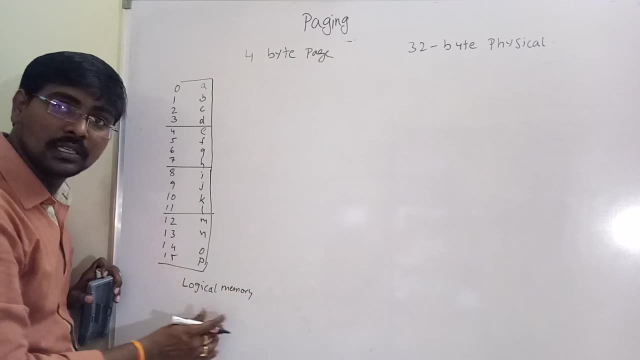 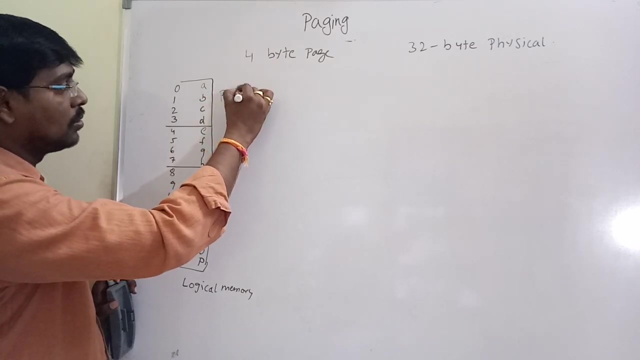 A L M N. Okay, This is the logical memory. Logical memory Consists of How many number of pages Here? this logical memory consists of 4 pages Here. size of This is page 0.. This is page 1.. 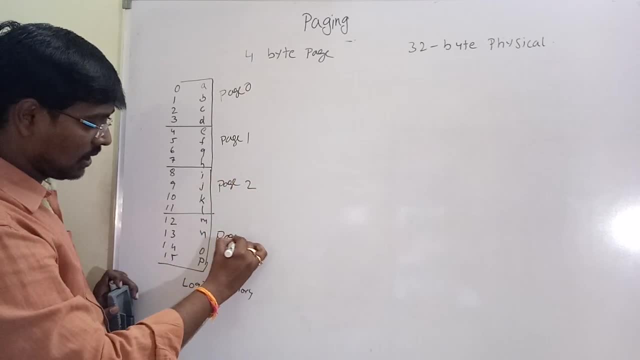 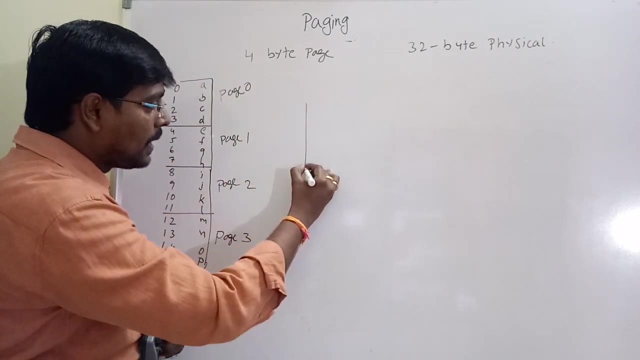 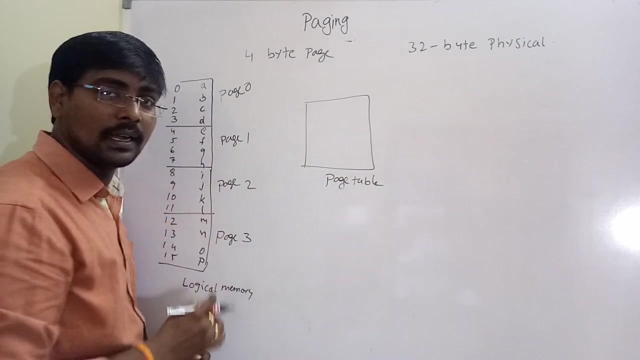 Page 2. Page 3.. 4 pages Here. size of each page is 4 bytes. Now Move to page table. Now move to page table. This is the page table. Page table contains The corresponding frame number, Suppose 0.. 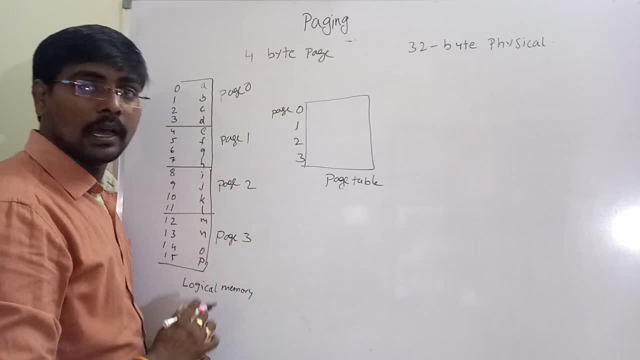 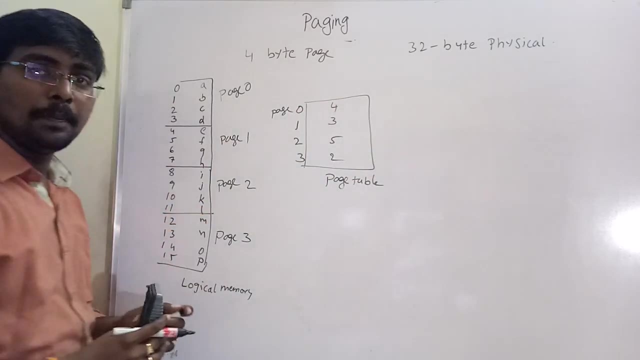 1, 2, 3. That is page 0. Assume page 0 is placed at position 4.. Suppose 3. 5, 2. That is the page 0. Is at frame number 4.. Page 1 is at frame number 3.. 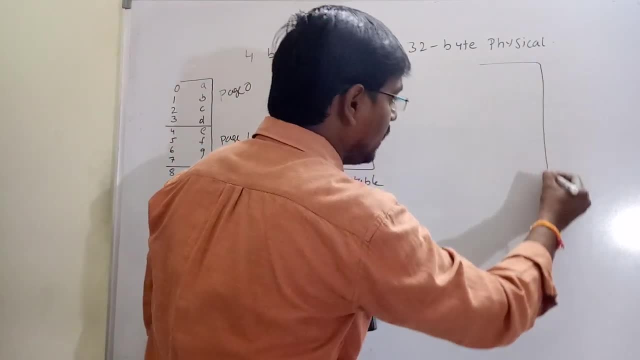 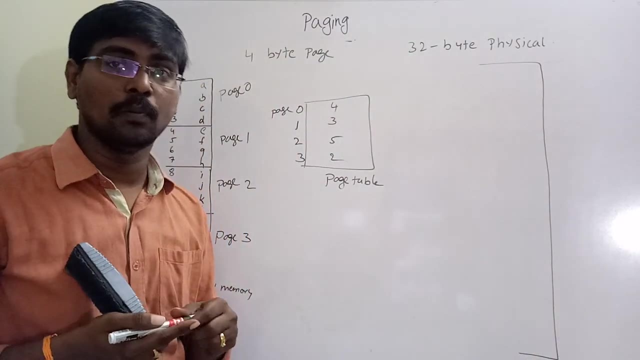 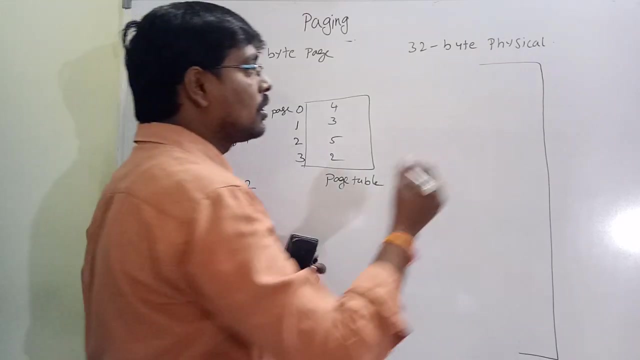 This is A 32 byte. This is a 32 byte Physical memory. Physical memory. Why I am using 32 bytes. The size of the page. The size of the page Is equal to the size of the frame, So compulsory. 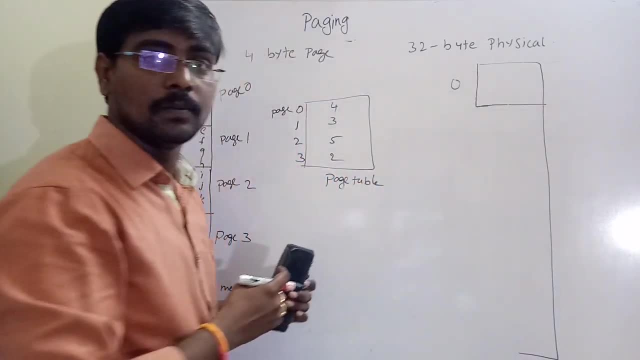 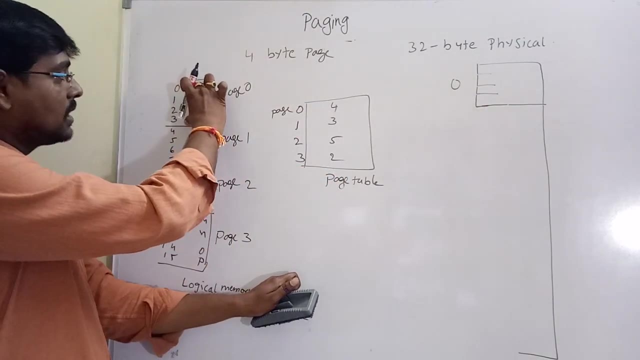 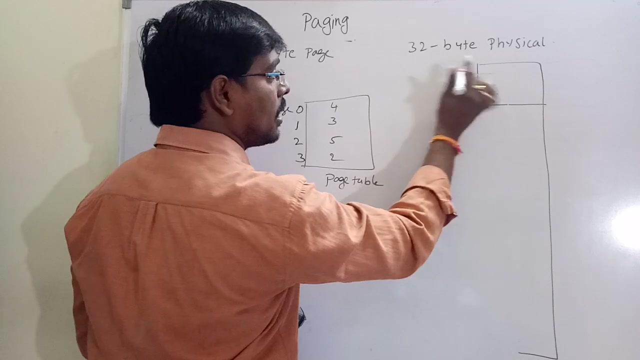 For example, Assume this is frame 0.. Frame 0.. How many parts it contains: 1,, 2,, 3, 4.. So here, Definitely, it also contains 4 bytes. It also contains 4 bytes. 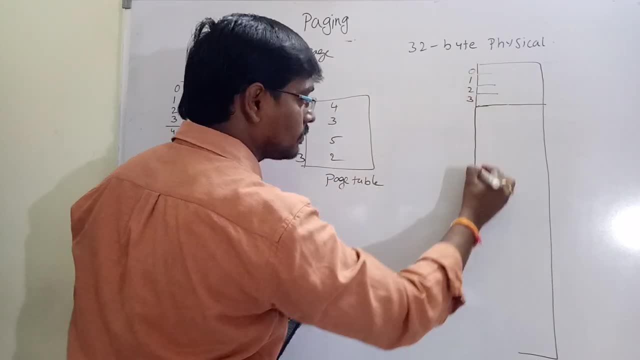 So I am writing as: 0, 1,, 2,, 3.. 4,, 5,, 6,, 7.. 4,, 5, 6, 7.. 4,, 5,, 6, 7.. 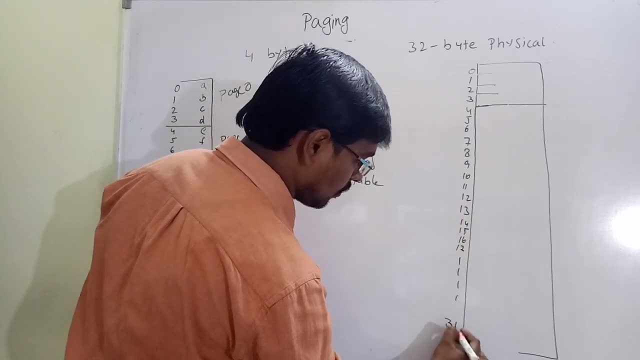 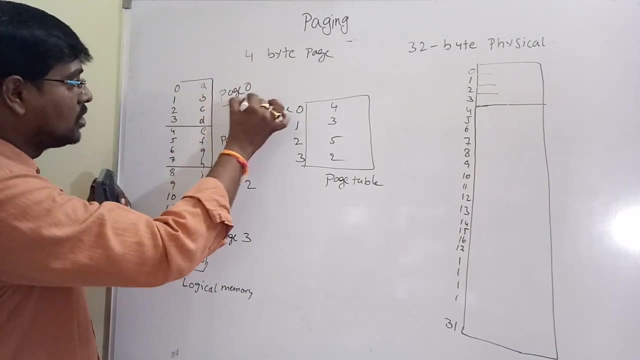 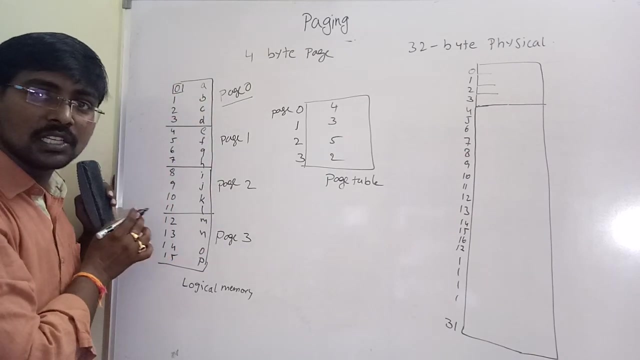 31.. 31. And so on: 31. How the operation is performed. Suppose: first page 0.. The logical address 0.. First page 0.. Where the logical address 0.. Is stored in the memory. Logical address 0.. 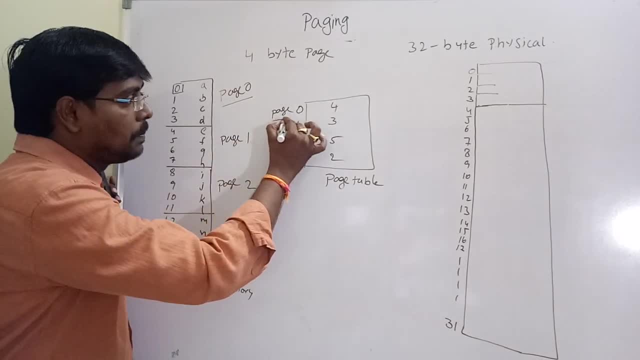 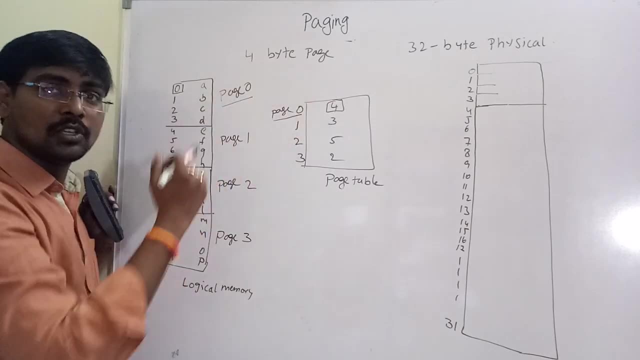 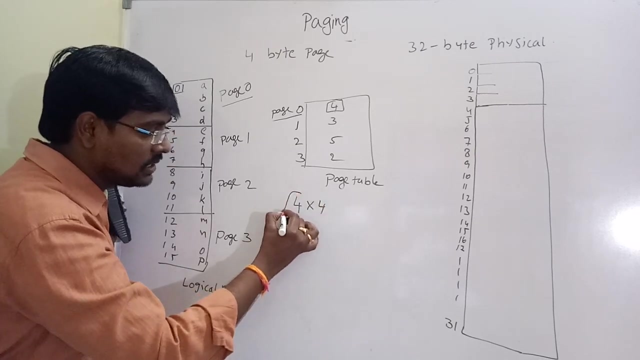 Is stored in the memory. So in which position? First, page 0.. The base address is 4.. Page 0. The base address is 4.. In which location The size of each page is 4 bytes, So 4 into 4.. 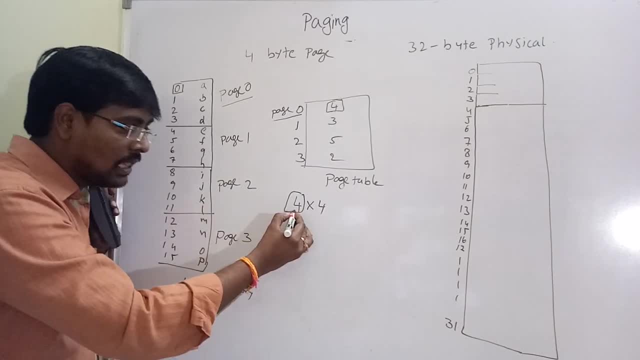 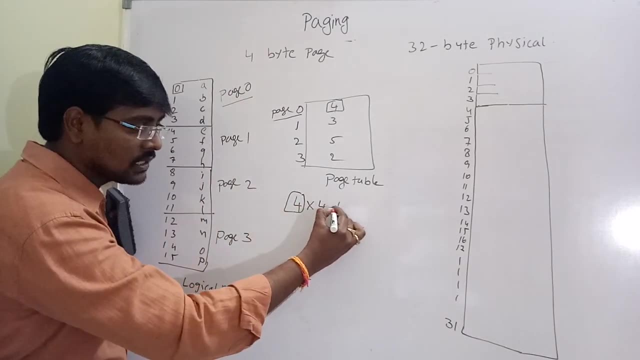 This is the frame number. The frame number is 4.. What is the size of each page? The size of each frame is 4.. So 4 into 4.. Plus offset is 0., So 0. That is at 16th position. 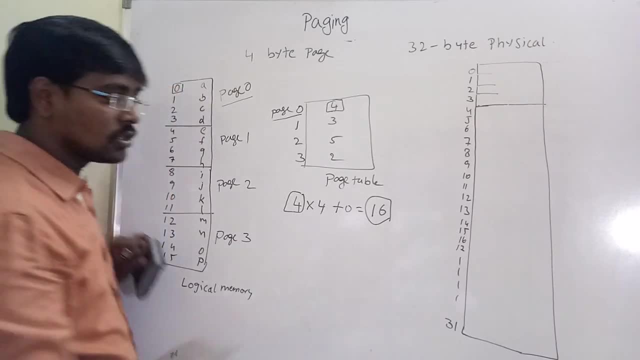 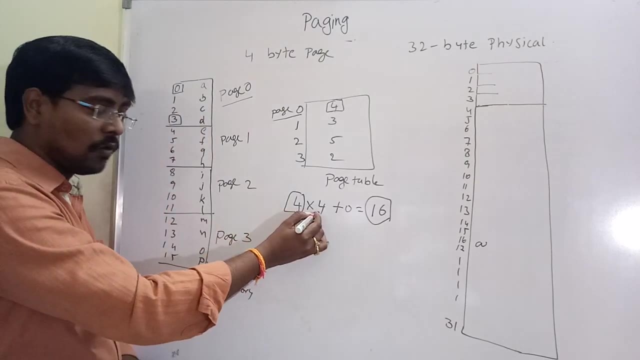 At 16th position. This A is stored. So this A is stored at 16th position. So this A is stored at 16th position. Suppose: 3. 4 into 4. Plus 3. 16 plus 3.. 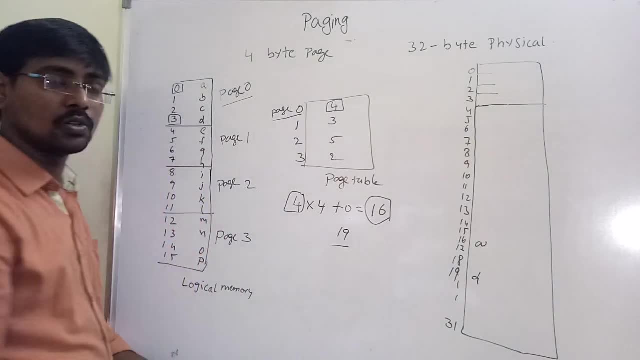 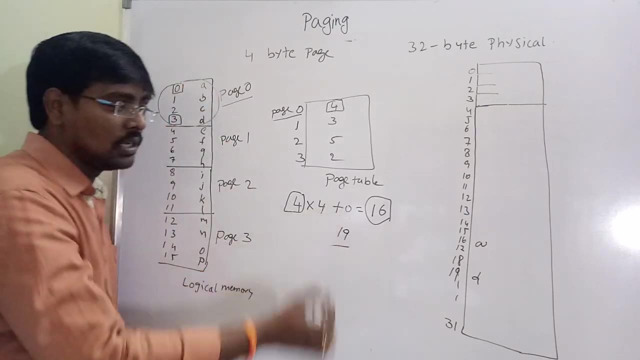 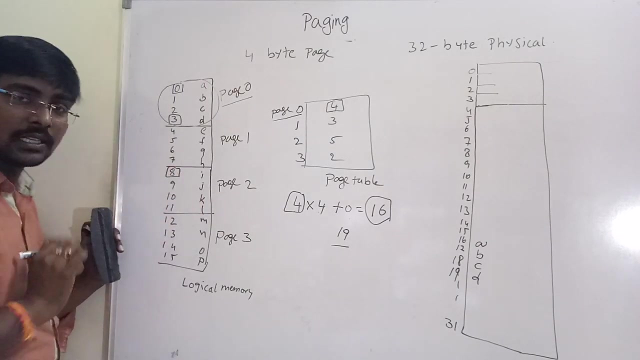 19. C, D is stored. Ok, All these are stored in a sequential. All these 4 are stored in sequential. All these 4 are stored in sequential: A, B, C, D. For example, consider this one: What is the place of the logical address H? 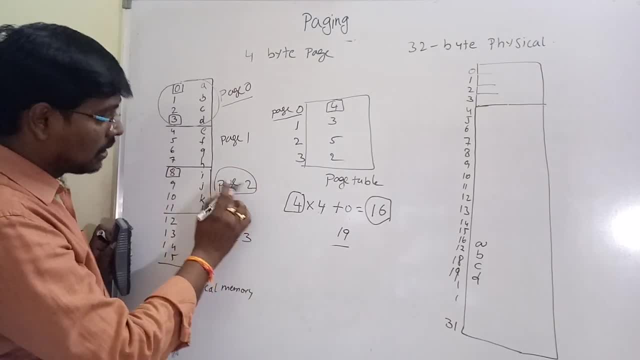 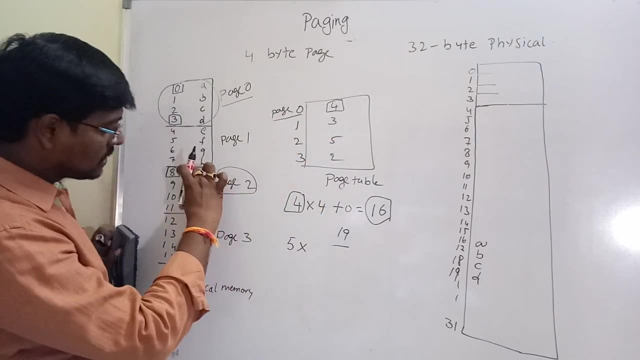 What is the place of the logical address H? First move to page number. The page number is 2.. What is the frame? number 5.. So 5 into Or size of each frame is 4 bytes. 5 into 4.. 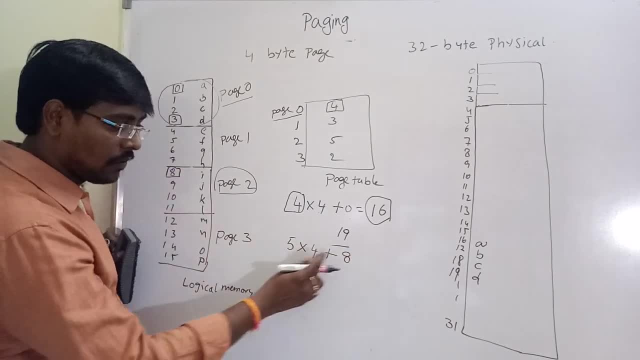 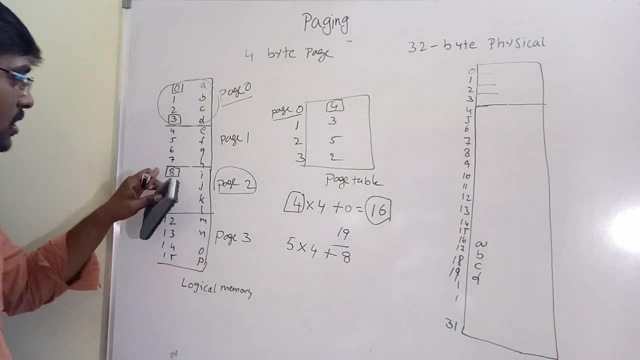 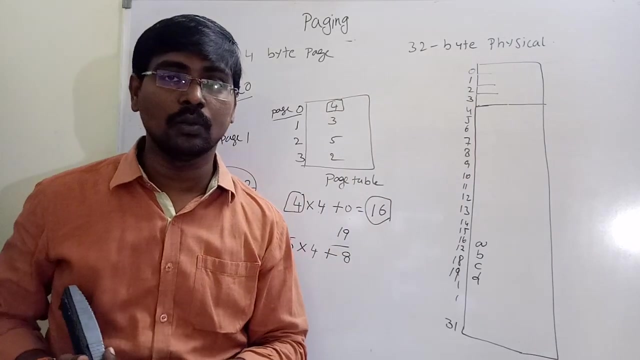 Plus offset value is H 5 into 4.. 20.. 20 plus H At the location 28.. This is stored. 29,, 30, 31.. 30, 31.. In this fashion, the pages are loaded into the frames. 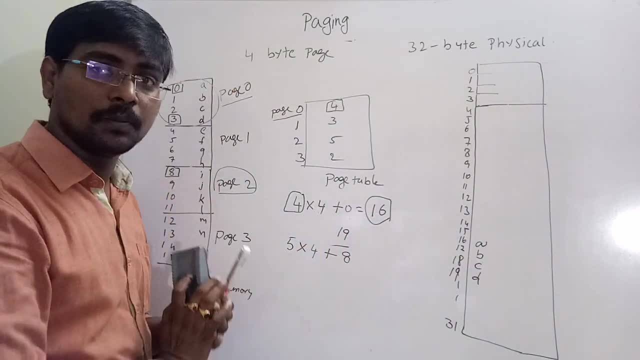 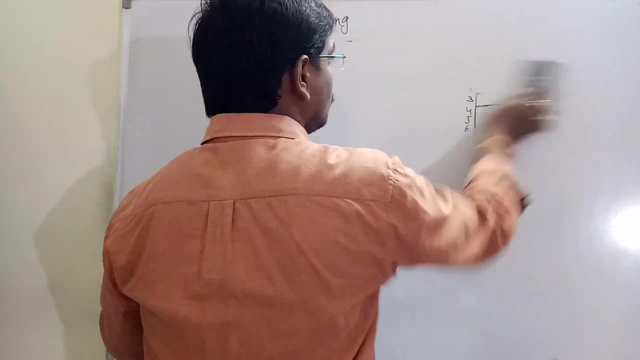 In this fashion, the pages are loaded into the frames. Ok, So this is a complicated example. No need to write. So now move to in the paging. So now move to in the paging. So now move to in the paging. Now move to the basic hardware. 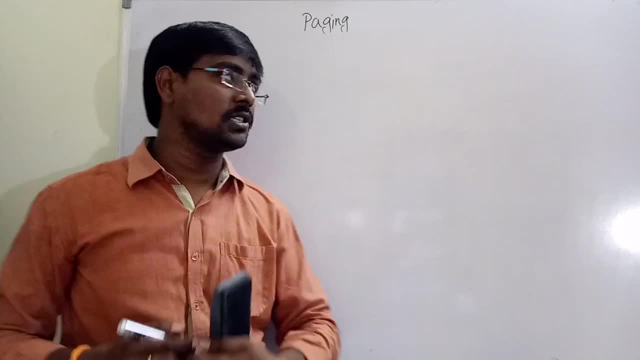 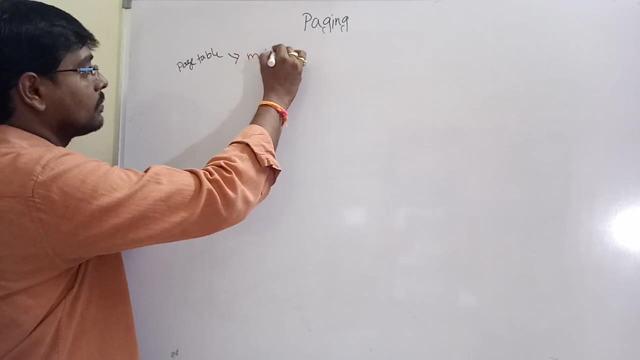 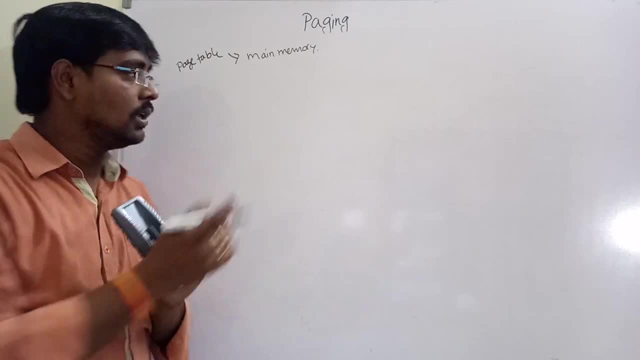 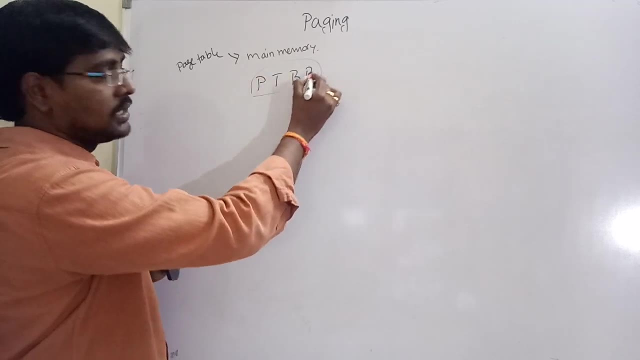 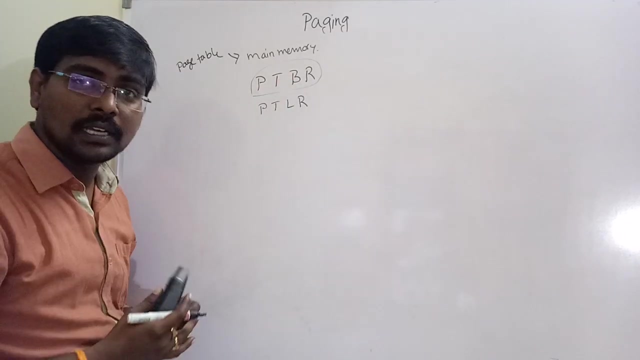 The page table is stored in main memory. The page table is stored in main memory. We are maintaining a page table base register. We are maintaining a page table base register: PTBR, PTBR, PTBR, PTBR, PTBR. 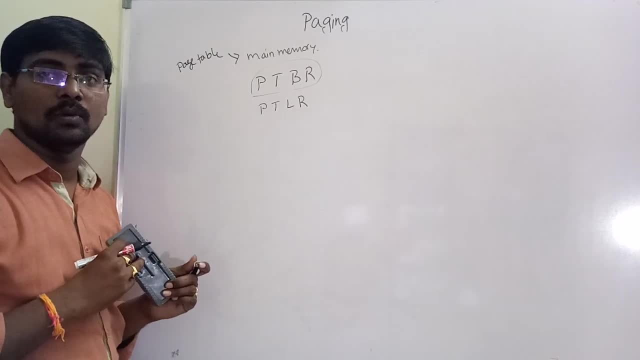 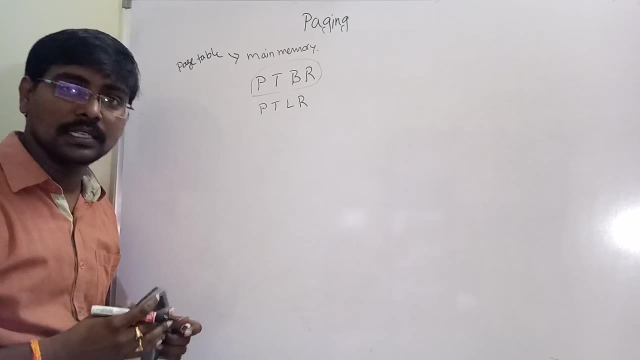 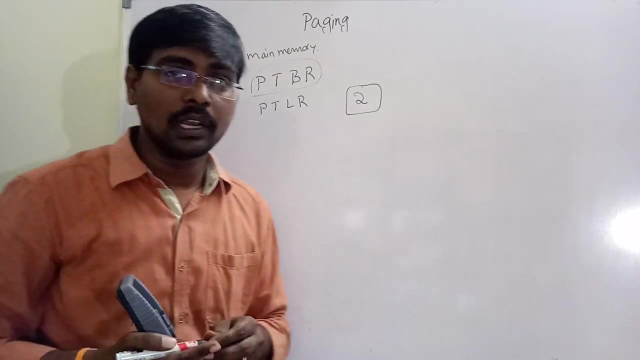 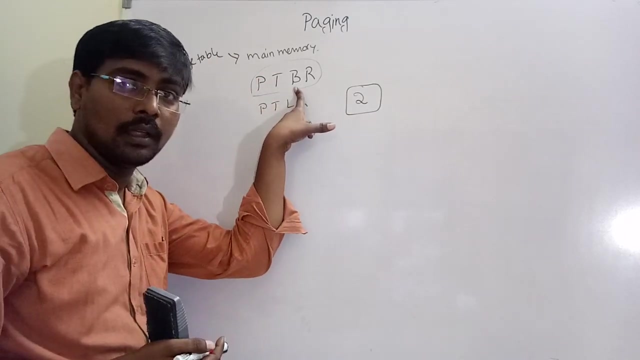 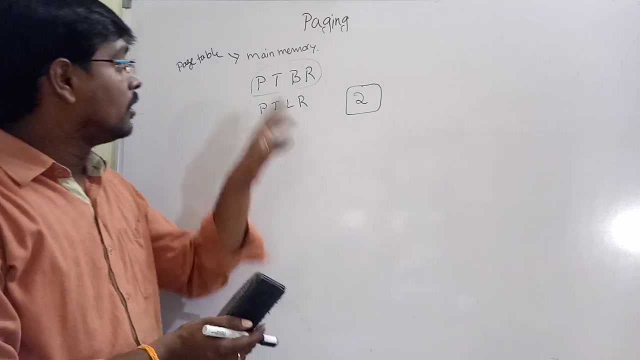 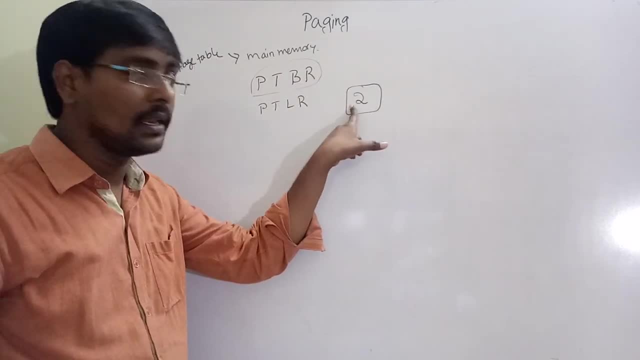 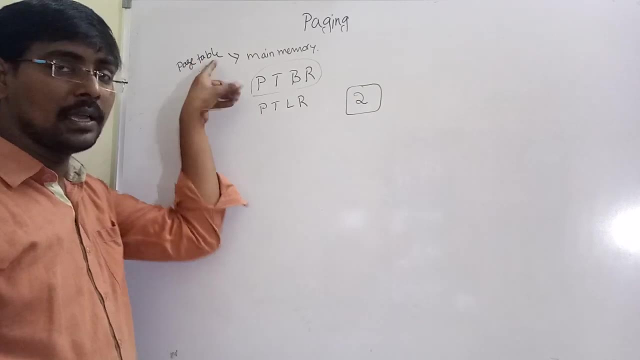 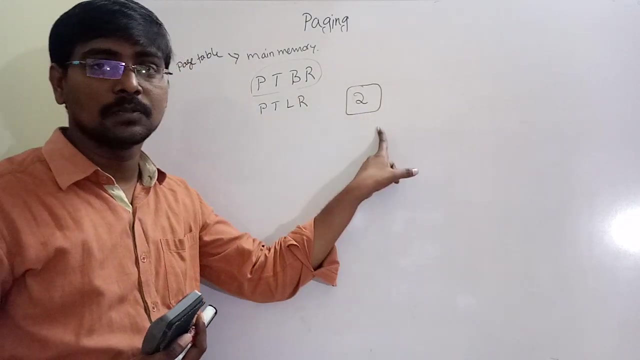 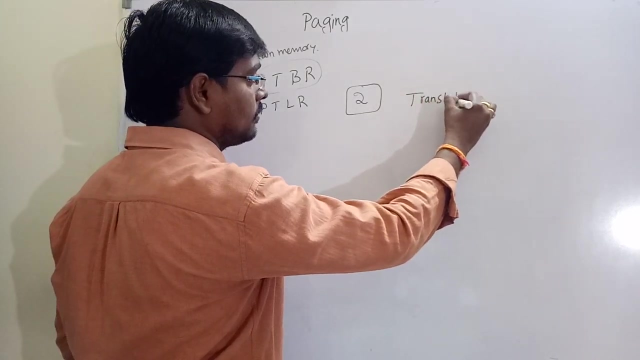 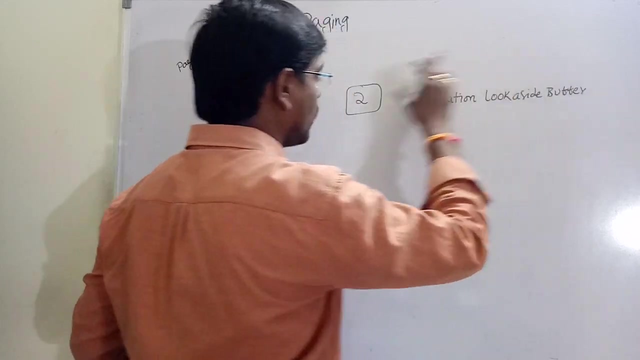 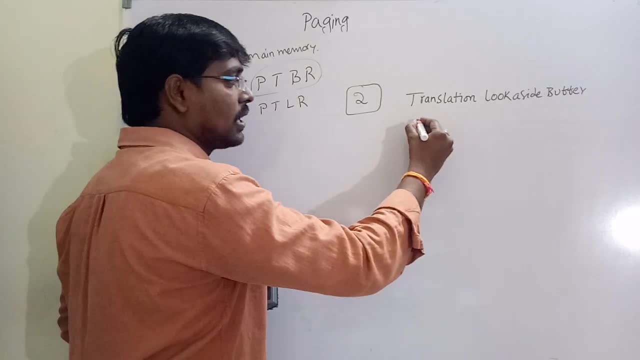 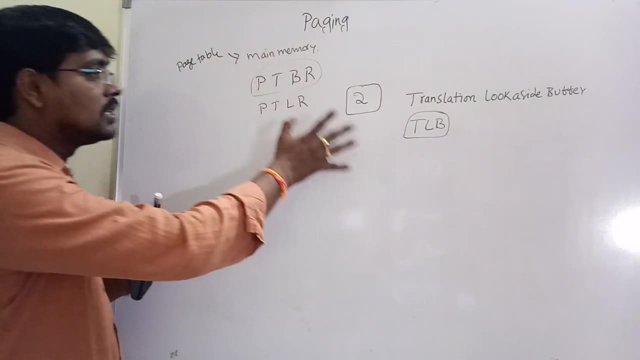 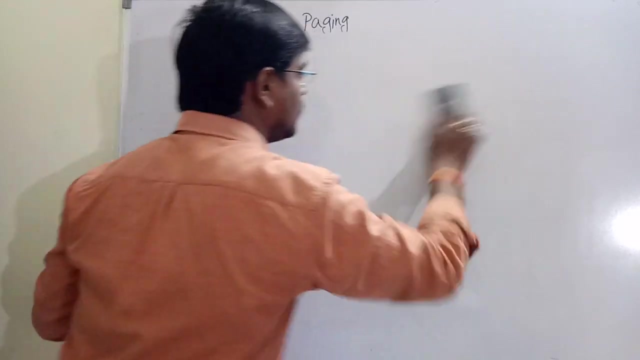 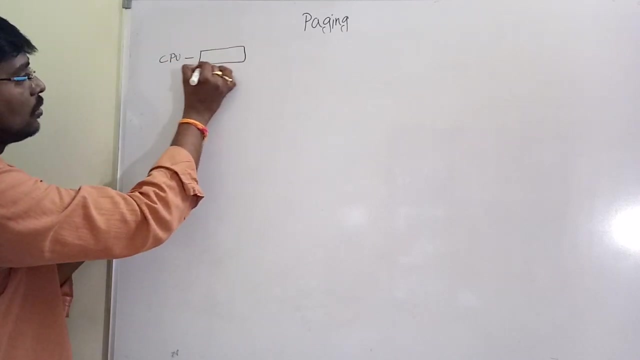 This is called a speed cashew translation. look aside: buffer TLP: How the operation is performed by using TLP. This is the important concept in paging How the operation is performed. First, the CPU generates the address. The address is divided into two parts, page number. 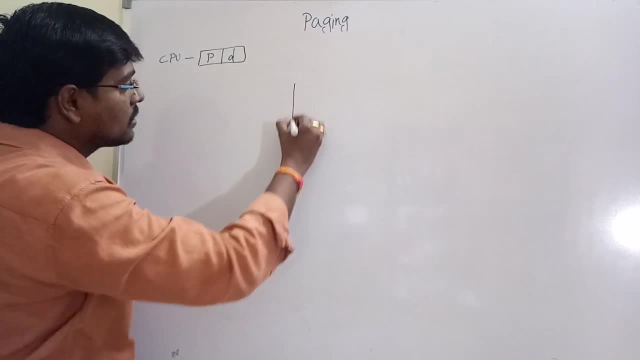 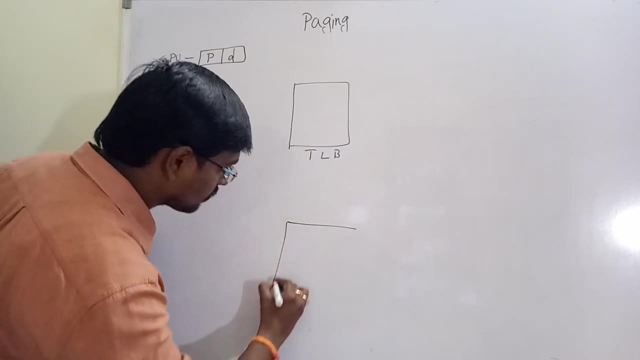 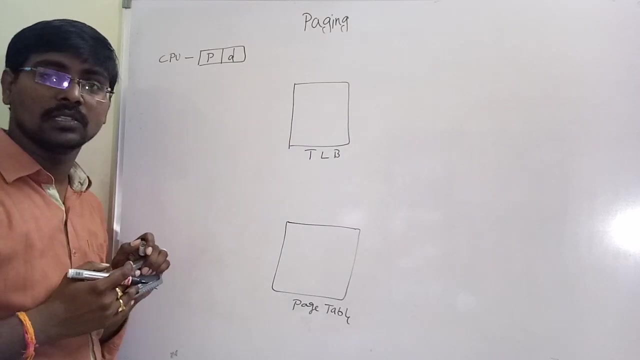 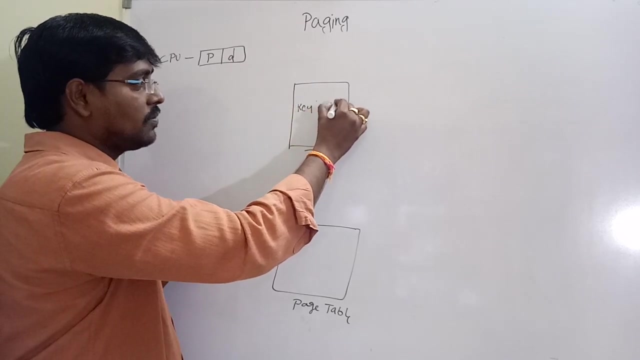 offset First. suppose this is translation. look aside buffer. This is translation. look aside buffer. This is page table Here. translation: look aside buffer contains what It contains two values. One is key or tag. Second, one is value. That means simply, it consists of the page. 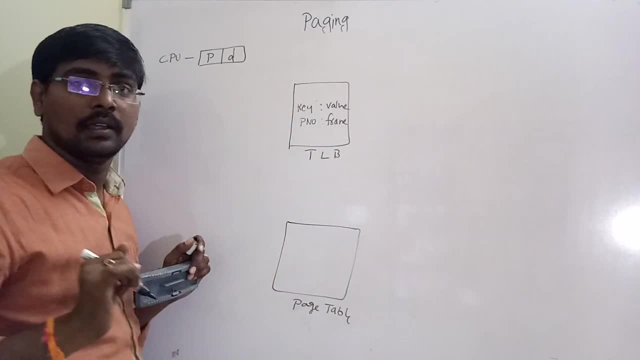 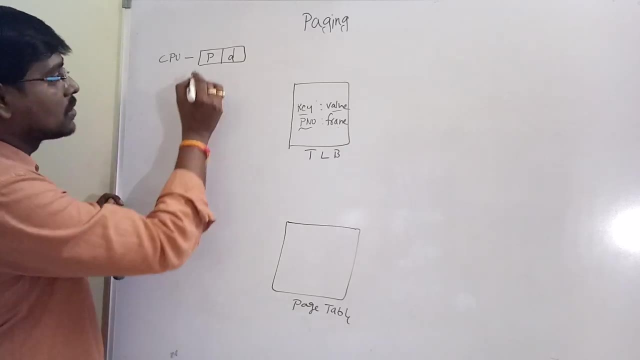 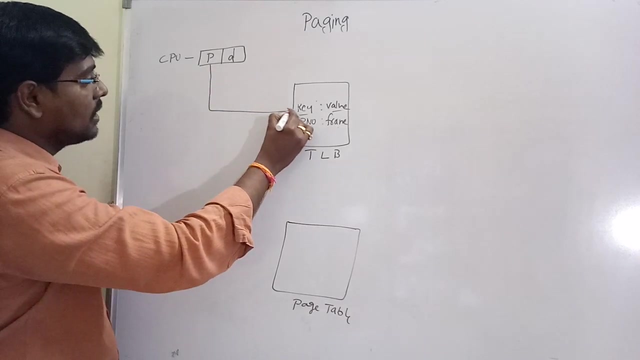 number and the corresponding frame number. Contains two parameters: the key and a value, That is, the page number and the corresponding frame number. See this one CPU generates the logical address First. this address is checked in the translation. look aside. buffer First our page number. 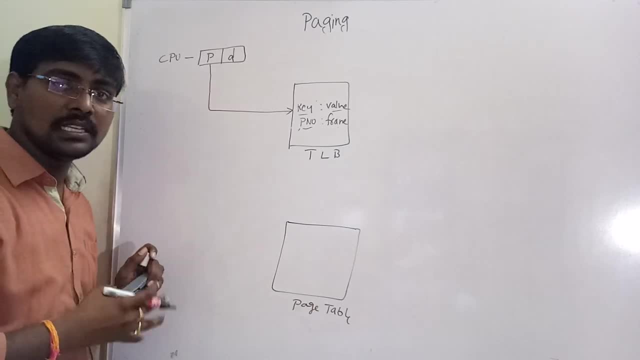 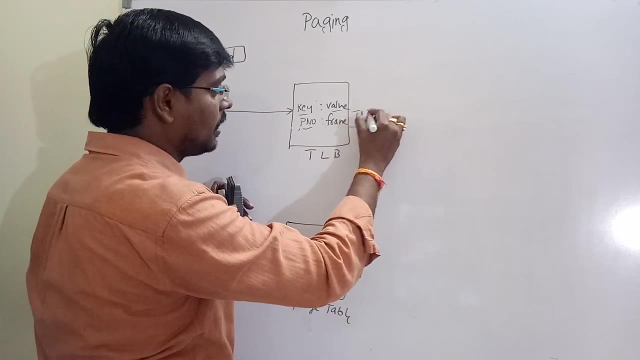 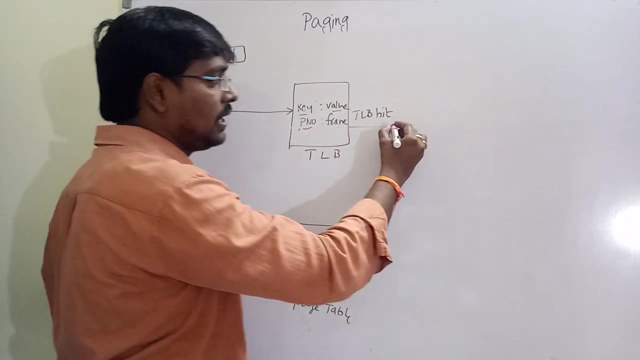 is checked in the TLP Suppose if our page number is available. if our page is available, that means this is called TLP hit. It means our required page is available in the translation. look aside buffer: Whenever it is available, what we will do- The corresponding page number. 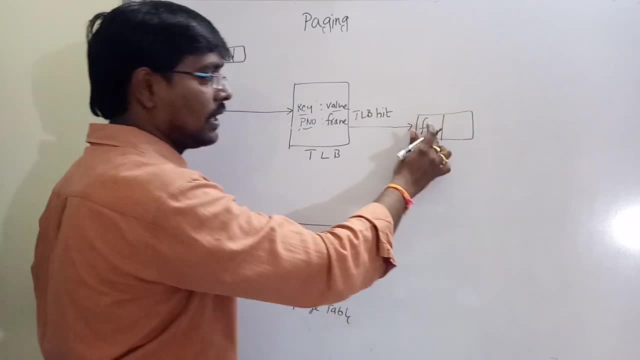 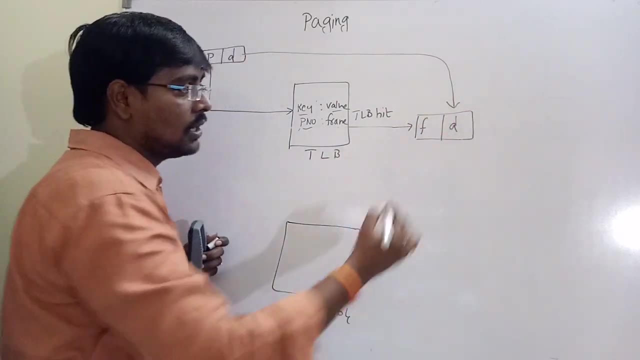 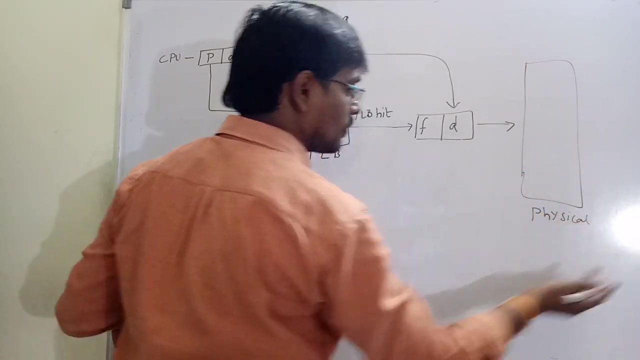 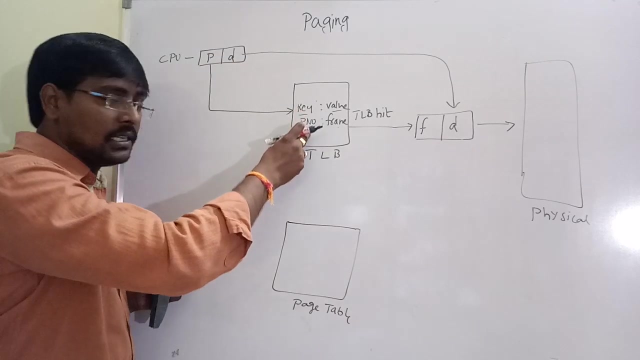 for the frame number or page number will be affected. We move to the physical memory list. We move to the physical memory list. For example, if the available frame- that is, the required page- is not in the TLP, or if the required page is not in the TLP, what we will do? We will change the frame number to the number. 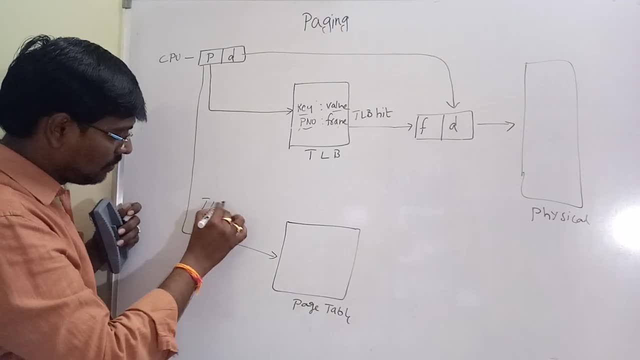 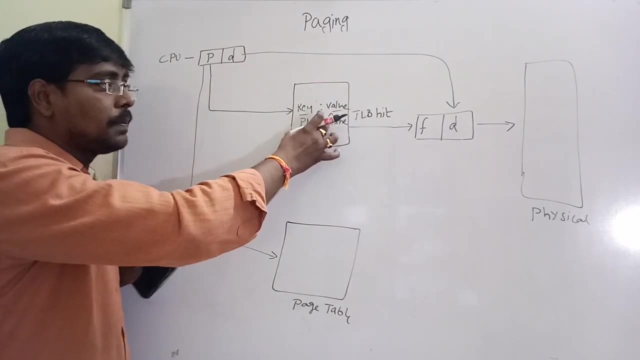 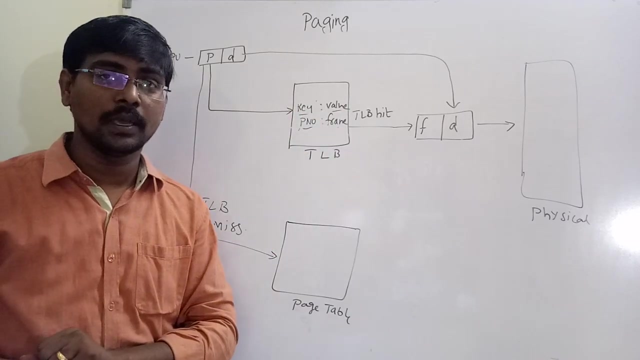 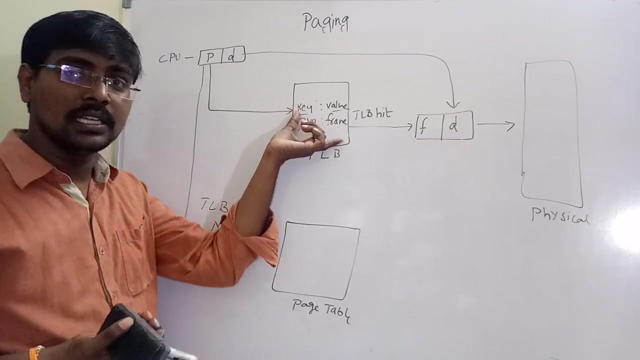 What we will do. that means TLB miss. that means always first we search the TLB if it is present. why this TLB is a cache? that means it contains only a limited number of pages. suppose if it contains 1000 pages, it contains only 100, searching from 100 is easy compared to searching from 1000, okay, 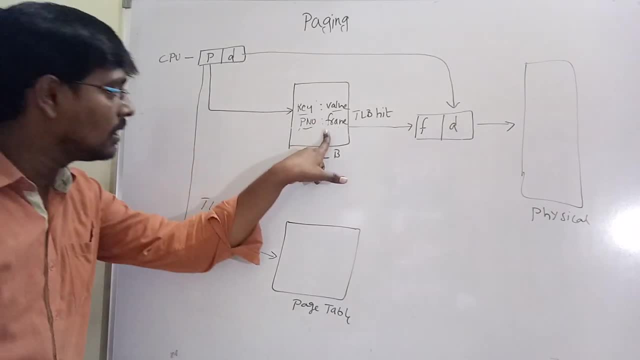 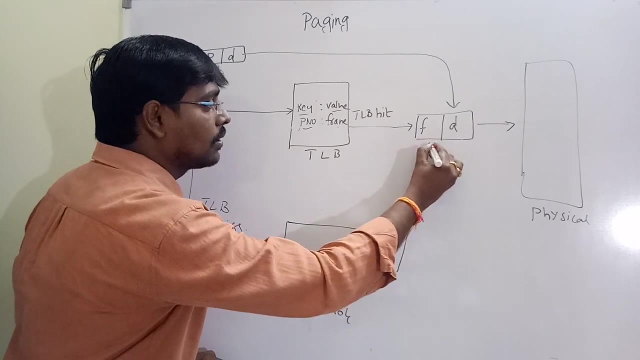 So TLB, miss, miss. if the required page is not in the TLB, we are check the page table. from the page table, we access the frame. from the page table, we access the frame and move to the physical memory. this is the procedure of paging. 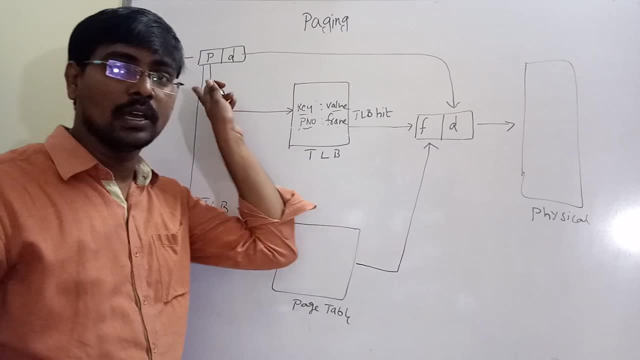 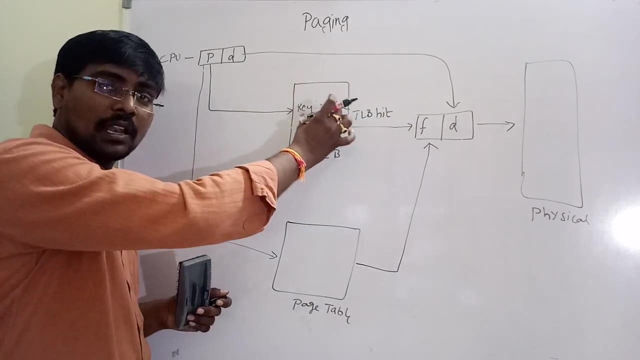 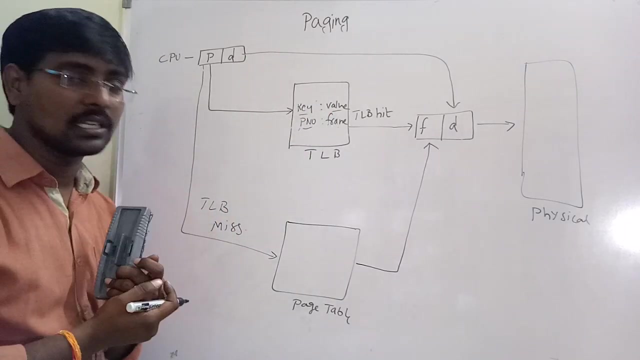 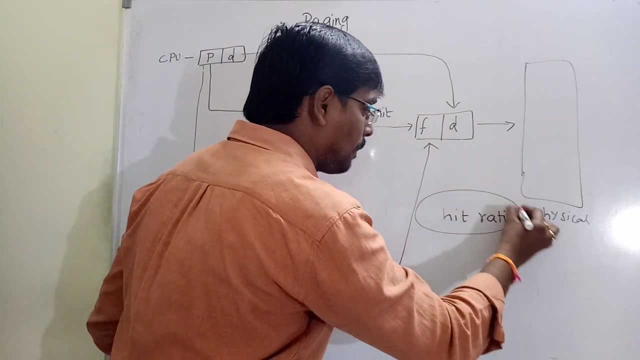 By using this TLB we are performing, that is, we are moving a page into frame Here: TLB hit miss. the page is available in the TLB. TLB miss means the page is not available in the TLB. that is the translation. look at it, for hit ratio means: hit ratio means the percentage of times our desired page is in the table memory TLB. 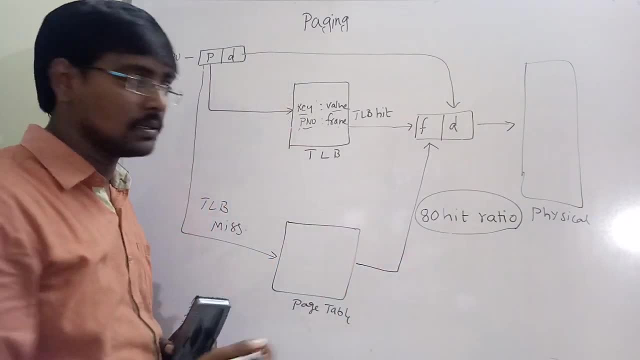 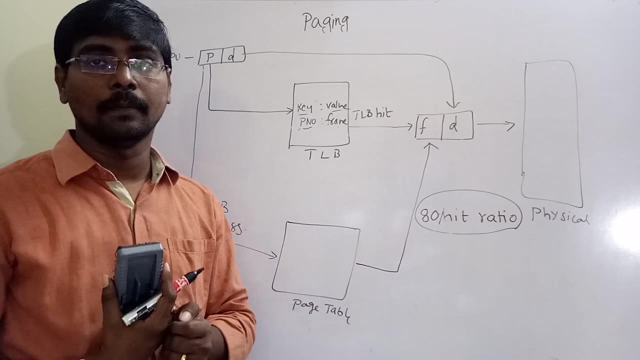 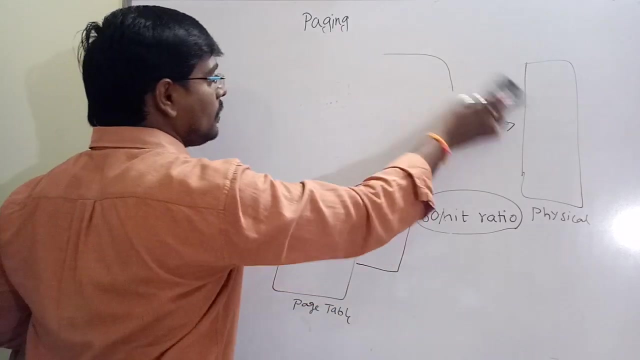 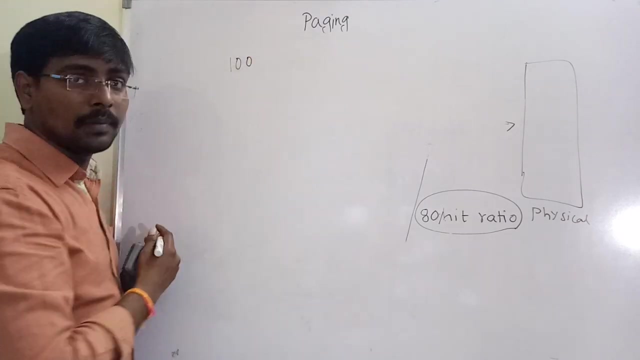 For example, 80% hit ratio means 80% hit ratio means 80% of time. our desired page is in the memory. our desired page is in the table memory. So TLB miss is in the translation. look at it buffer, For example. assume for each memory access of the TLB, for a memory access, we require some 100 MB. we require some 100 MB. 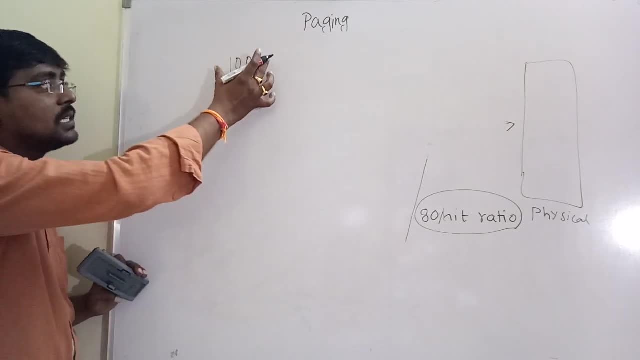 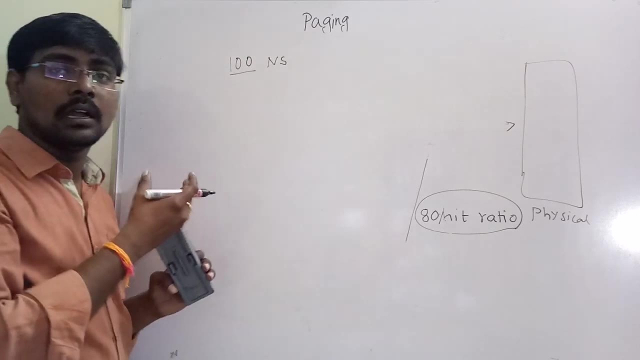 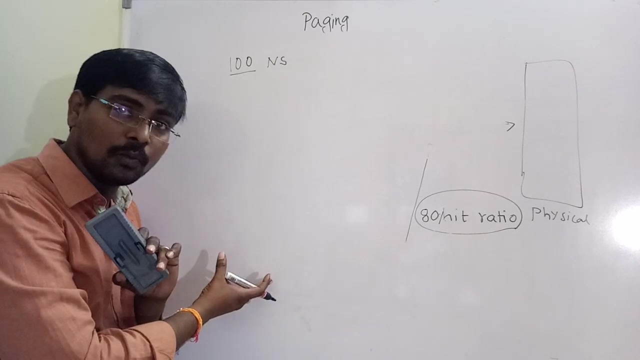 If the element, that is, if the page, is present in the TLB, it requires some- only 100 nanoseconds. What happens if the page is not available? If the page is not available, first we have to move the page table. we have to move the page table. before moving the page table, first we search in the TLB. 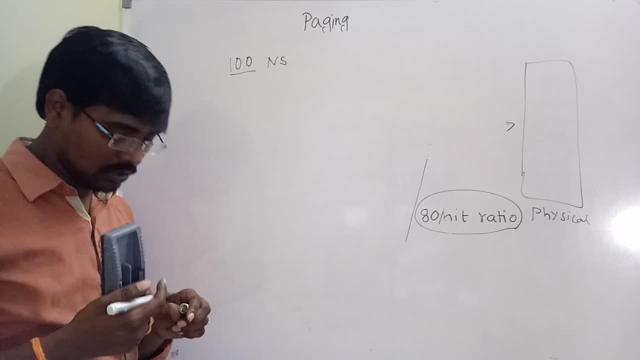 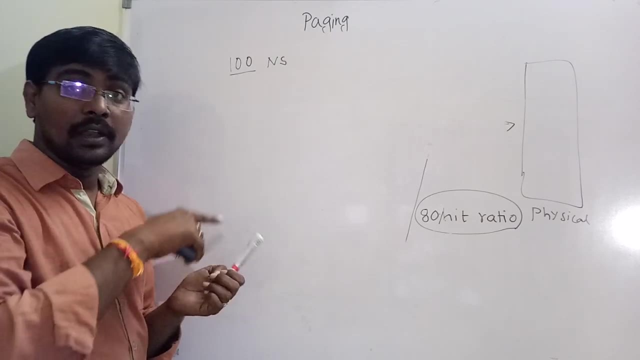 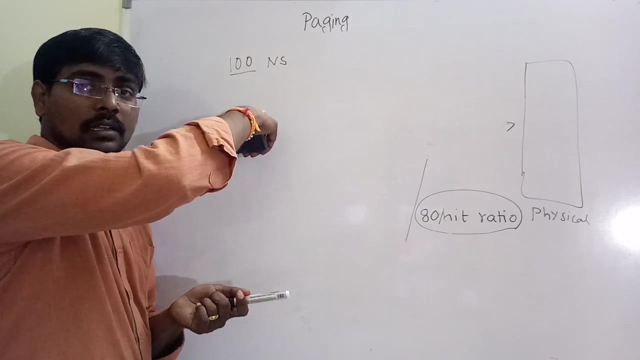 That means it requires a total of 200 nanoseconds. You got the point. To search for an item in the TLB, it requires 100 nanoseconds Whenever TLB fails, that is element is not in the TLB. that means we access but search, not present. 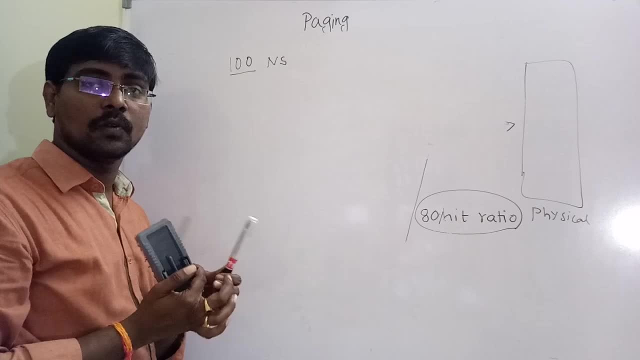 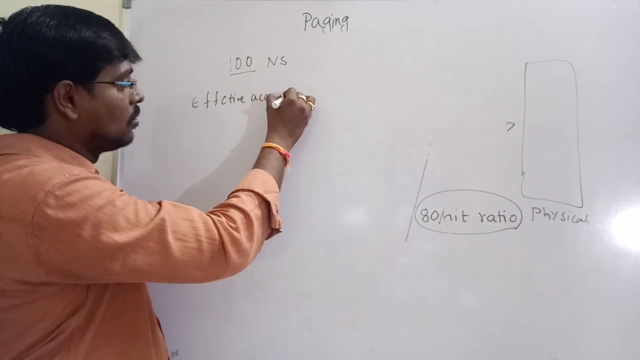 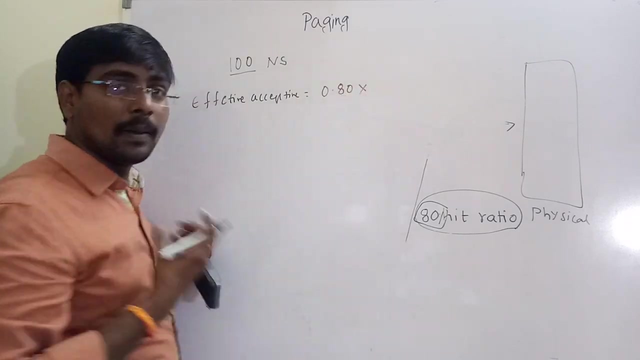 And go to the main memory, that is, the page table. again, it requires one more 100.. Simply effective access time is equal to, for example, if 80% miss the probability, 0.8, memory access time, that is, from the TLB, the memory access time is 100. 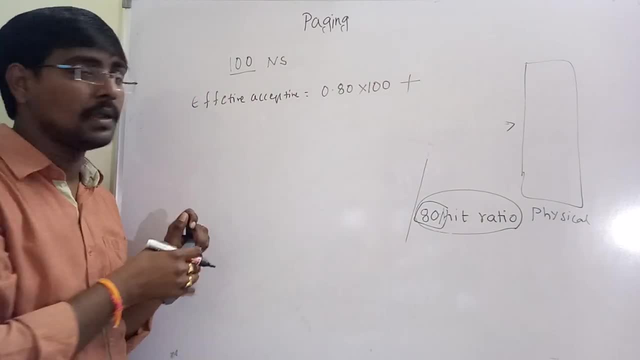 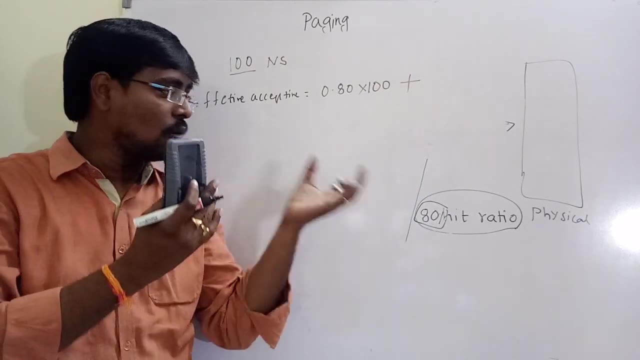 R means plus. this is the probability. R means plus. this is the TLB hit. TLB miss means total access time is 200 nanoseconds. one is for accessing the page table, another one is for accessing the required instruction. 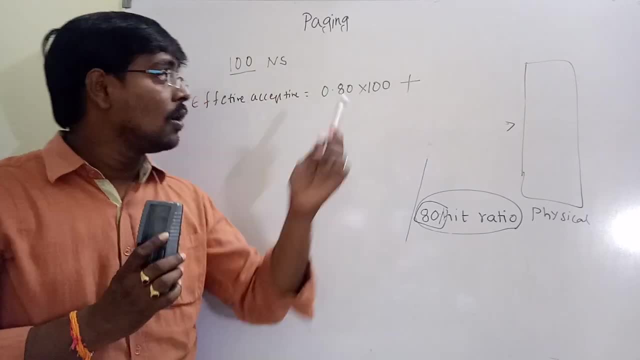 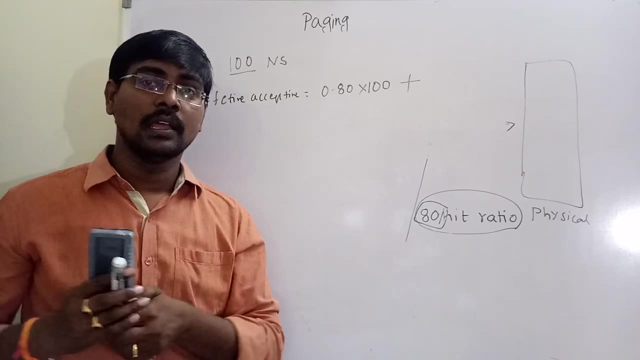 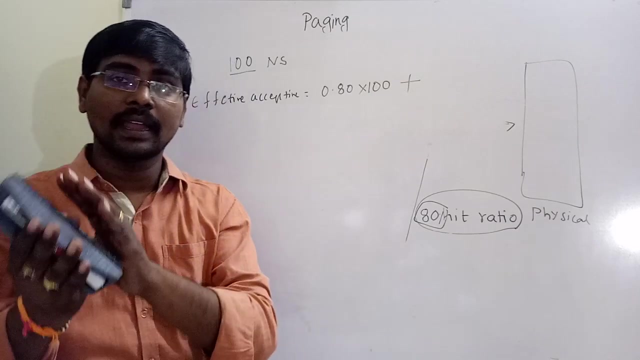 Before TLB: before TLB: I mentioned the point. what is the need for TLB? Suppose, if you want to access an entry, if you want to access an instruction from the page table, we required two memory access: one is for page table and another one is for instruction. 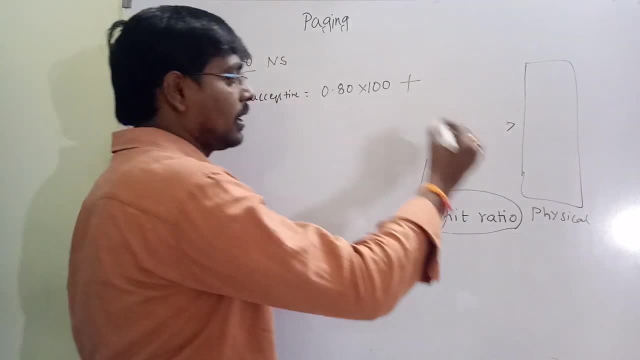 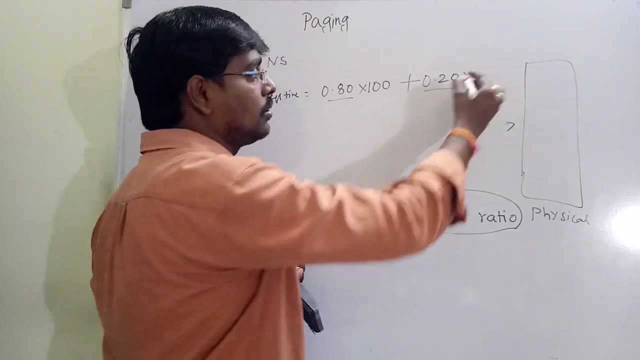 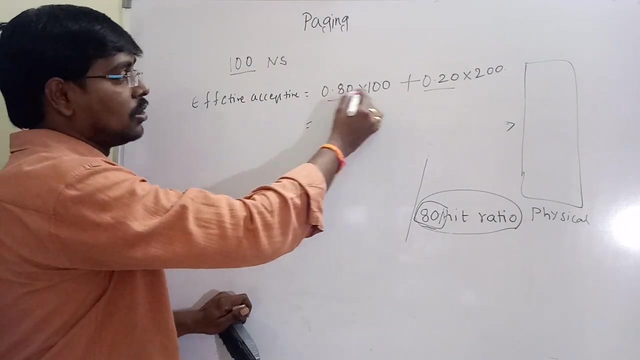 So 200, 2 into 100, 200 nanoseconds. the fail probability means 0.20, it is 0.8, means remaining value is 0.2.. So this is the value. suppose what is the value we are getting? 0.82, 80 plus 40, that is 130.. 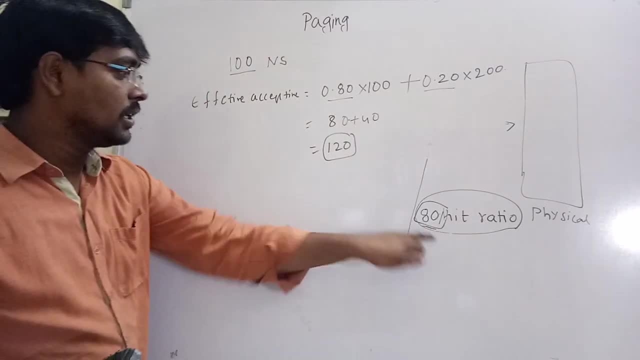 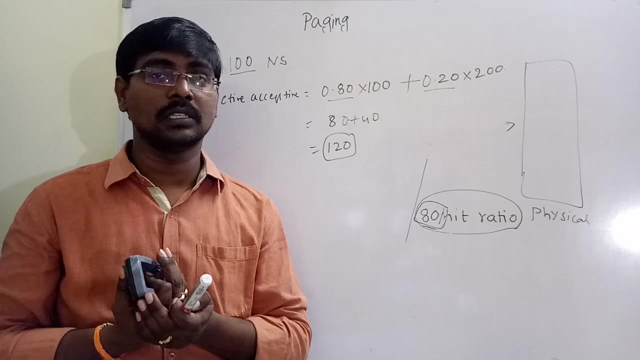 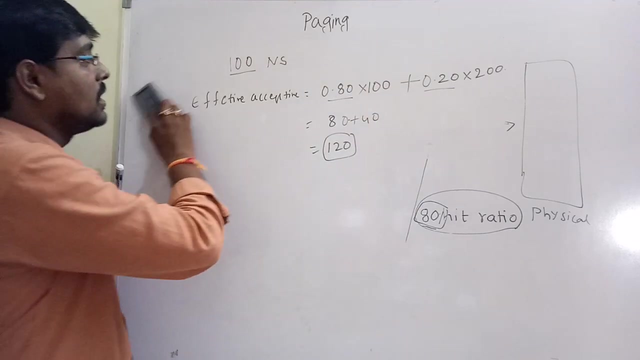 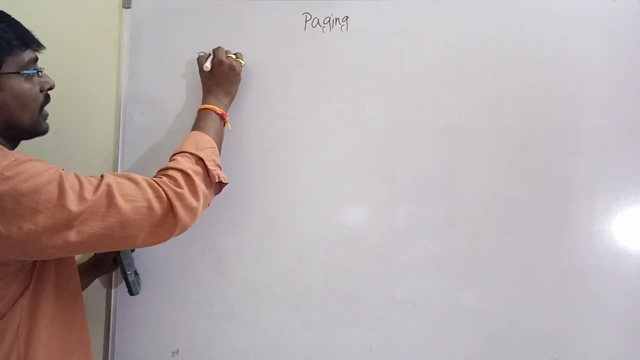 See this one: 80% hit ratio means the average memory Memory access time is 120, that is, it lowers the performance. that is, 20% of the performance is lower. okay, this is hitting In the paging concept. we have two more additional points. one point is protection. 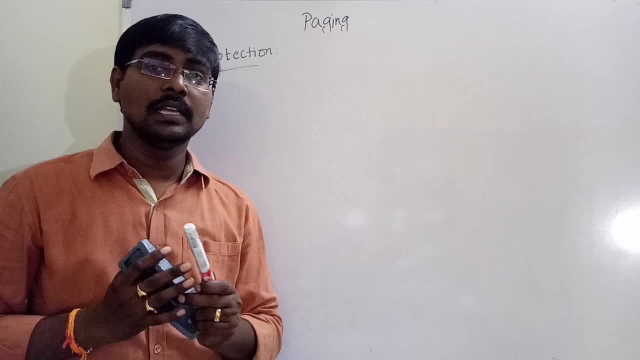 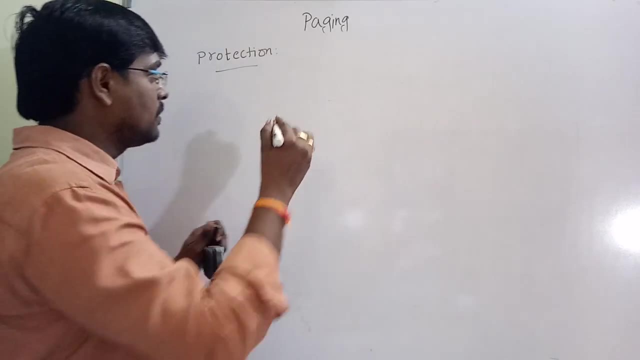 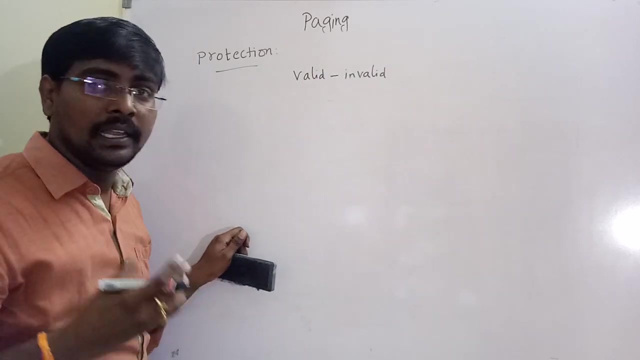 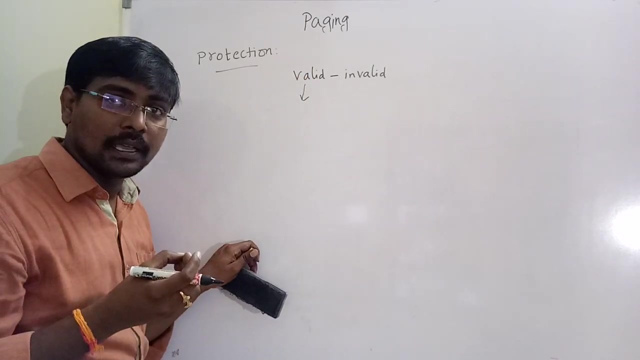 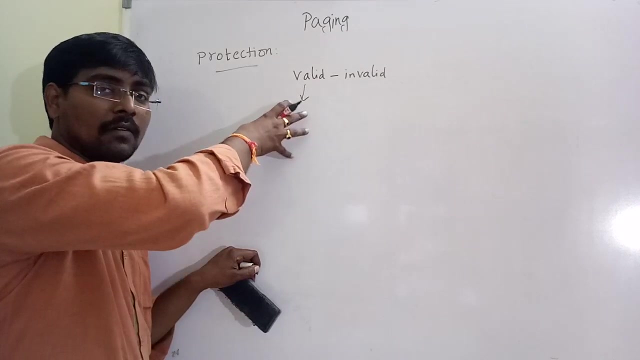 So this is the complete paging environment. in this paging environment we are providing protection to the frames. We are providing the protection to the frames by using valid invalid bit. By using valid invalid bit, we are providing protection. Valid means if the associated page, if the page is in the particular process, that is simply, if the page is available in the associated process, that is valid. 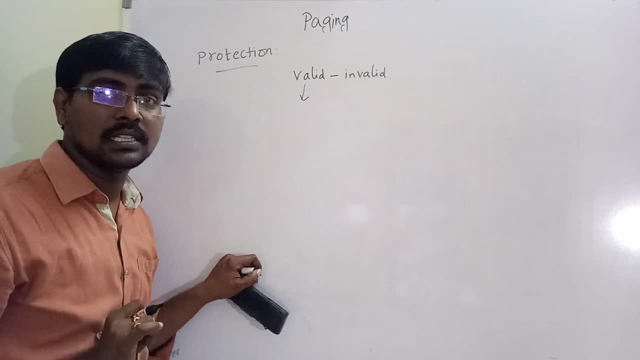 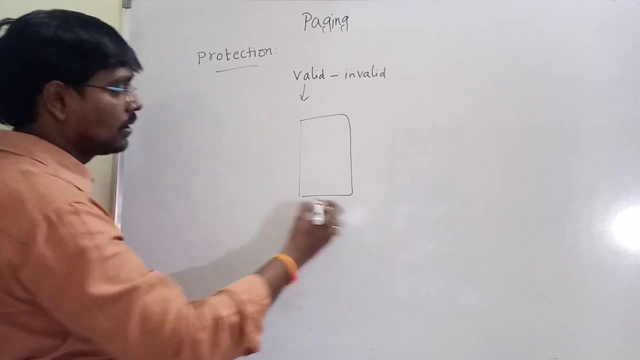 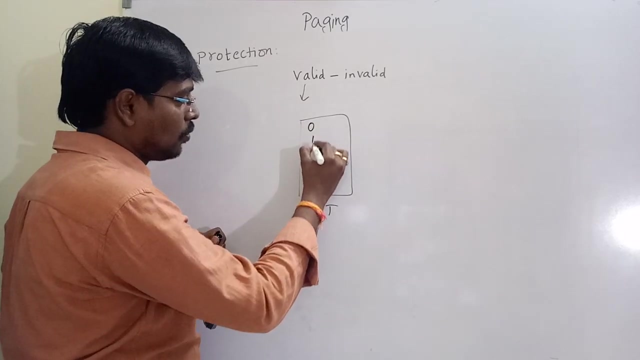 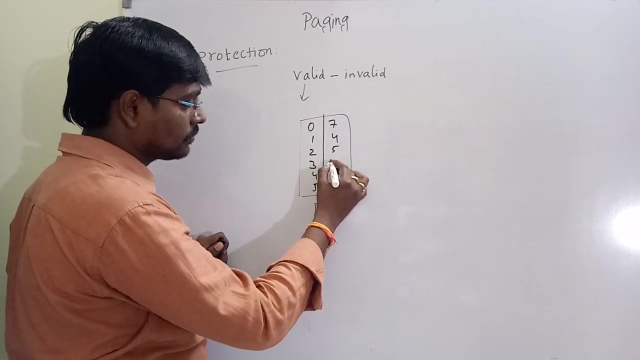 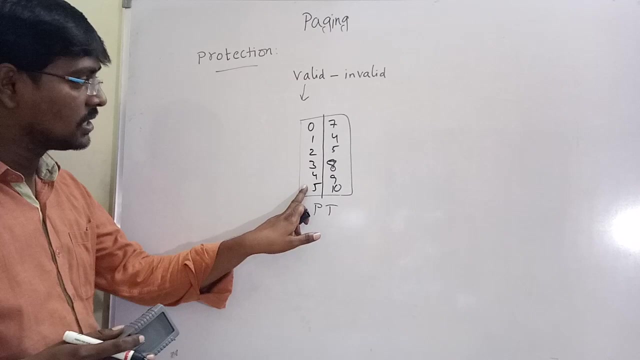 if the page is not in the process, that is invalid. simply see some example. suppose this is the page table. this is the page table. in this page table i have some pages, suppose the page 0, 1, 2, 3, 4, 5, 7, 4, 5, 8, 9, 10. in this way we are allocating the memory, so suppose this is the page number. 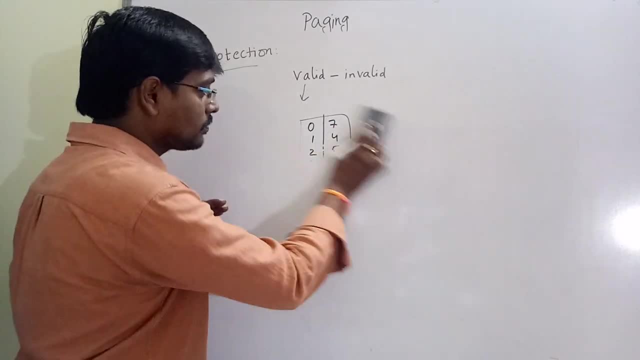 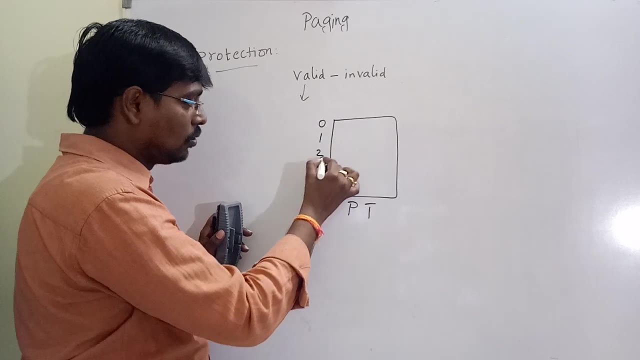 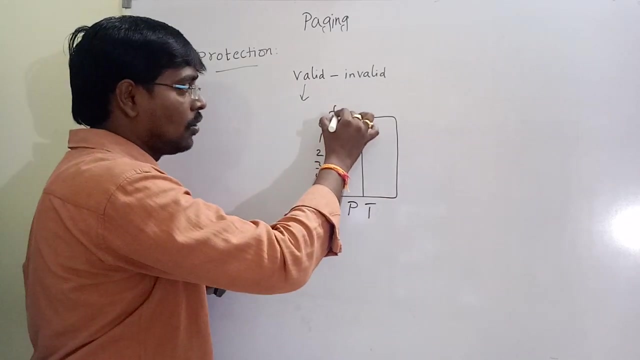 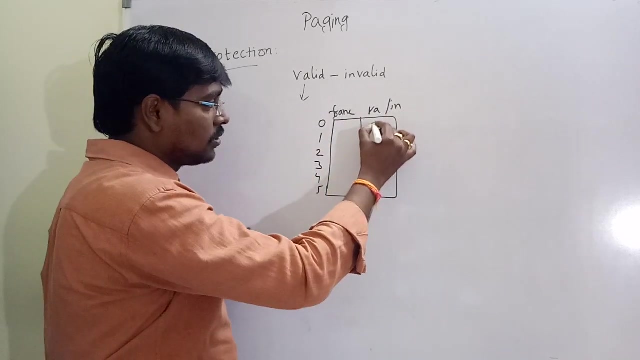 this is the corresponding frame numbers. assume, assume in this page table: 0, 1, 2, 3, 4, 5. these are the pages. this page table is now divided into two parts. one is the frame, another one is valid invalid bit. valid invalid bit suppose: v, v, v, i, i, the meaning. 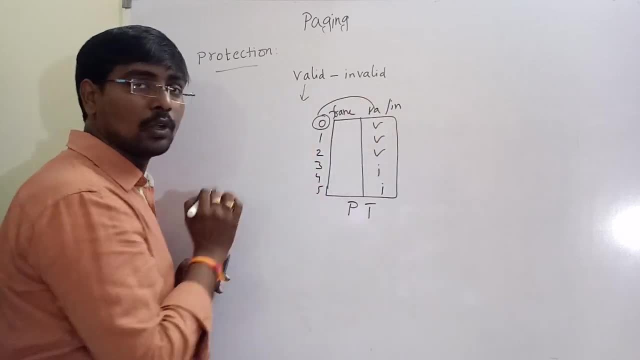 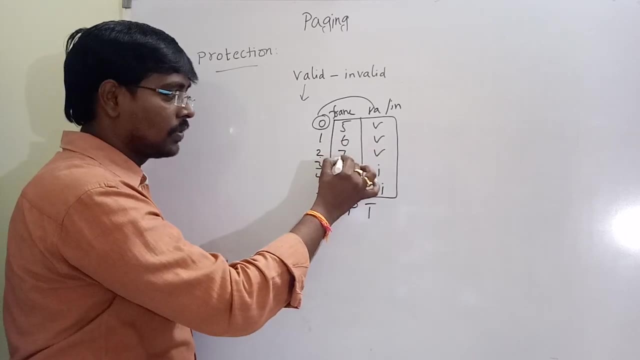 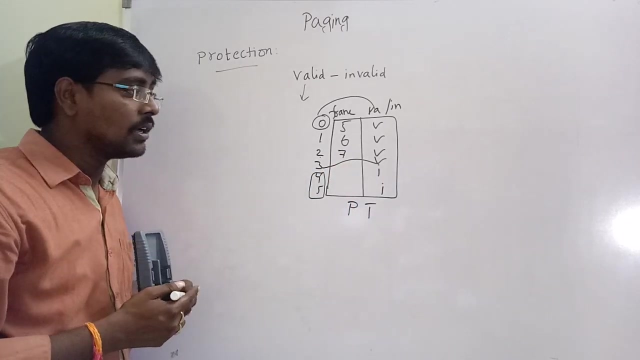 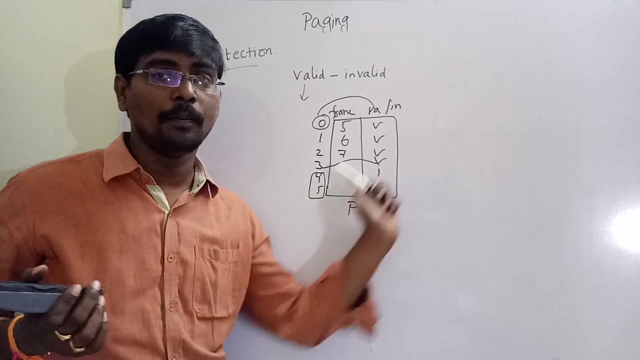 of this one is: page 0 has a particular frame, suppose frame number 5. page 1 has a frame. page 2 has a frame. suppose page 3 also has a frame. 4 and 5 are not valid. that means these pages are not in the associated process. but this 4 and 5 has no memory in the. that is no space in. 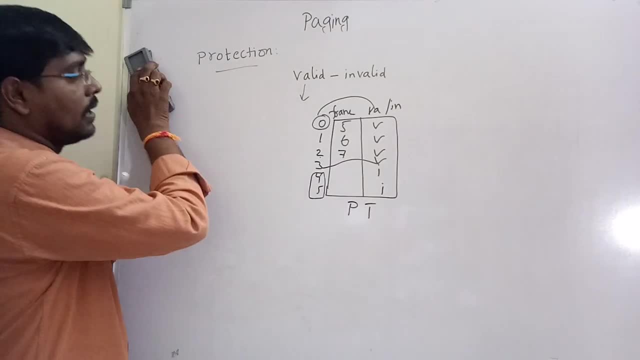 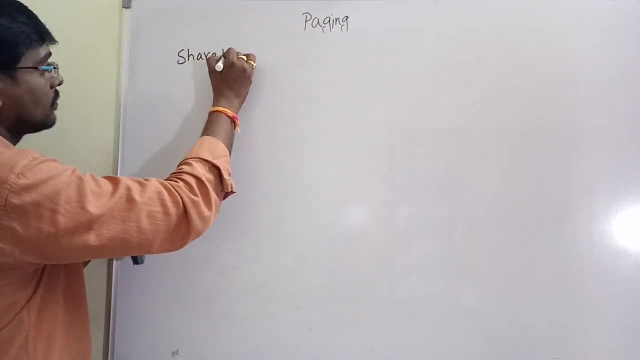 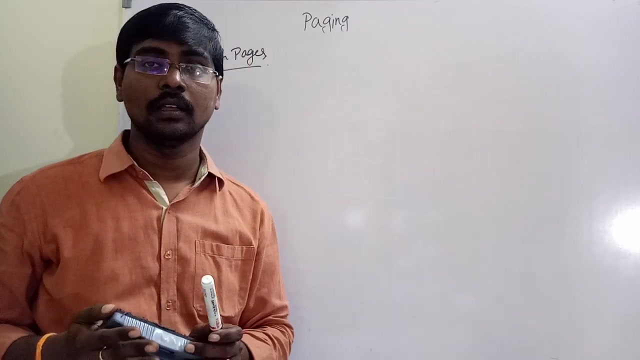 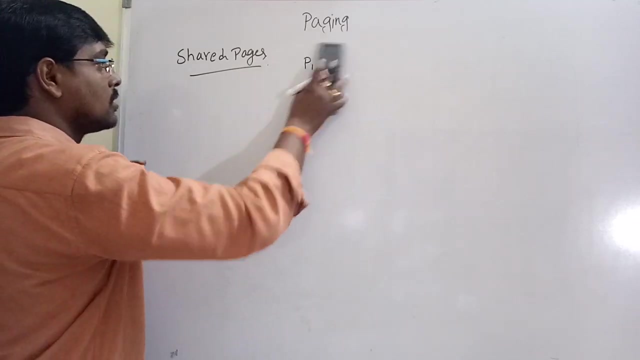 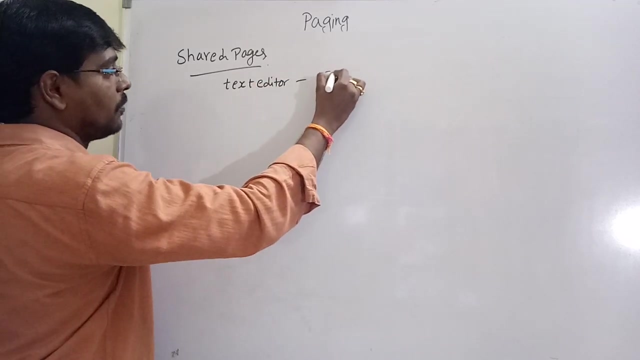 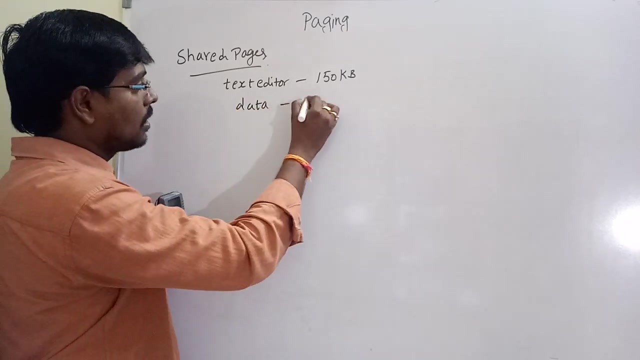 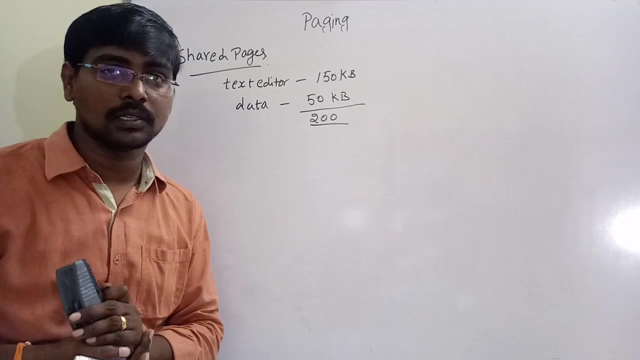 the physical memory. this is protection. and the last point we will discuss is on shared pages. the main advantage, that is, one of the advantage of paging, is sharing. sharing means. consider example. For example, we have three processes. First, we have a text editor of size 150 KB Suppose a data space of 50 KB. So total how much space required. It requires 200 KB of size. 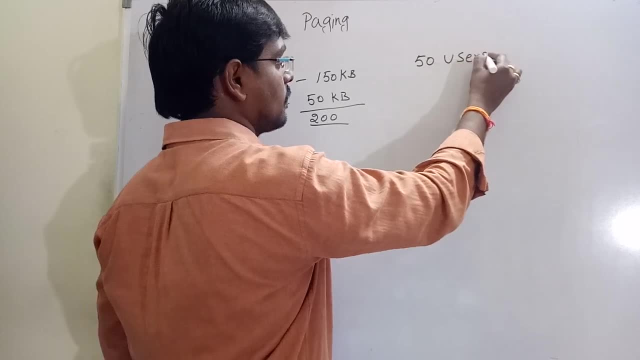 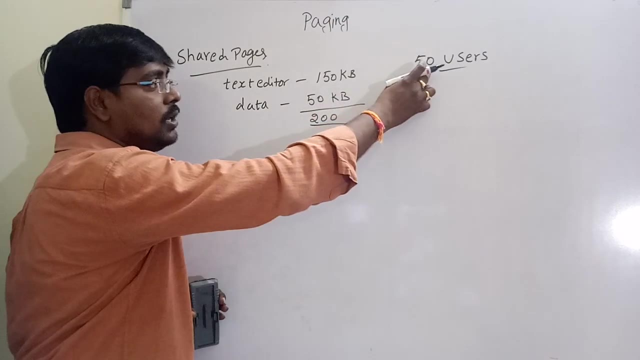 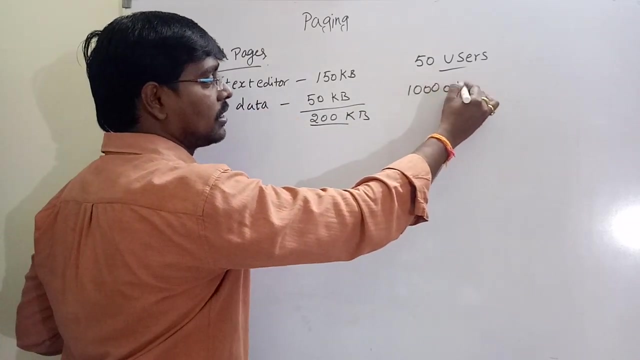 For example, if you have 50 users- Assume if you have 50 users, that is 50 processes- How much amount of memory is required? 50 users For each single user, it requires 200 KB. For 50 users: it requires 10,000 KB. It is clear. 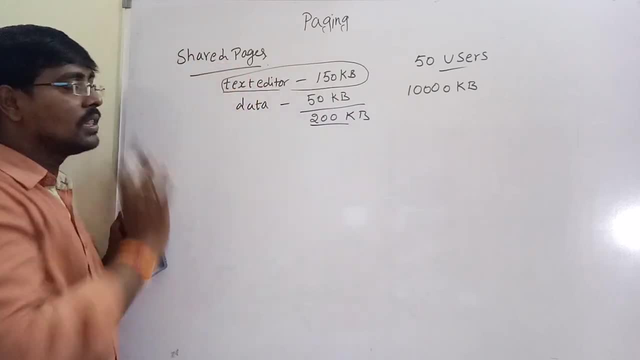 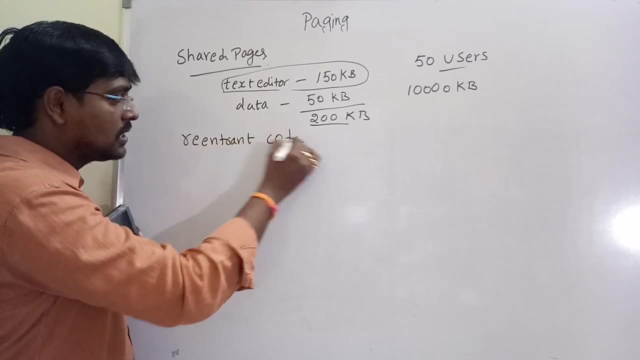 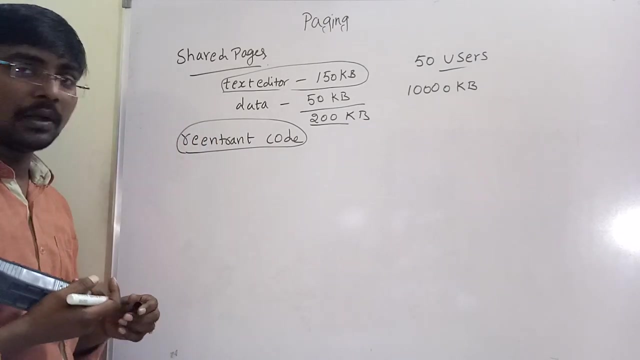 Assume this text editor. the code in the text editor is a reentrant code. Reentrant code is the code that is not modified, The pure code. that is the code not modified. More than one process at a time. execute the particular code. 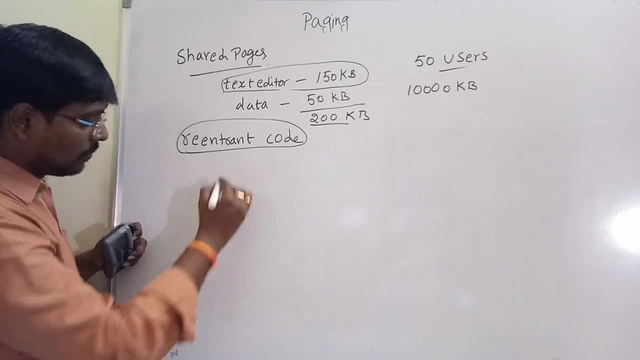 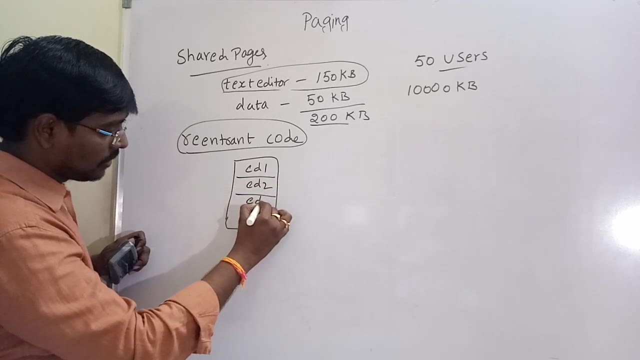 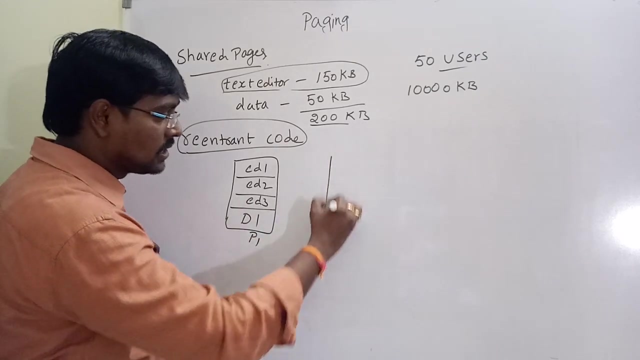 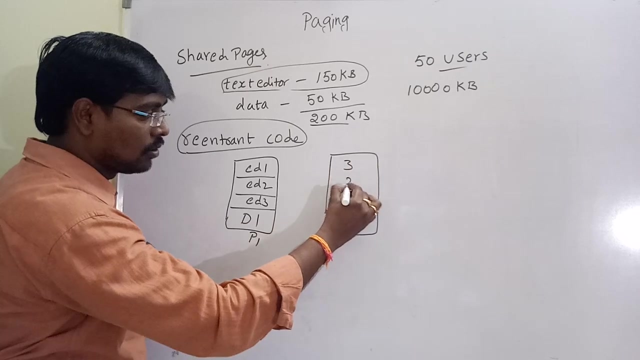 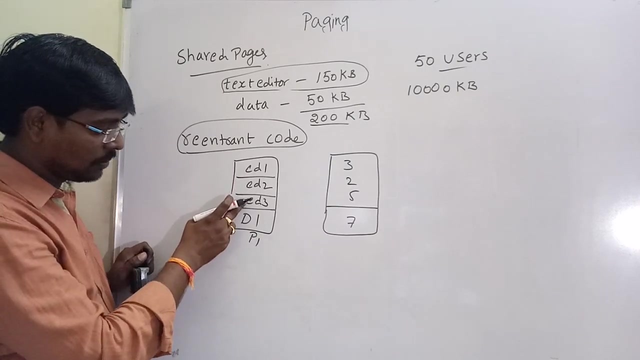 At a time. execute the particular code. For example, see this one: ED1,, ED2,, ED3.. Suppose D1.. For example, this is a process P1.. Assume process P1.. D1. This is the page table. This is the page table. In this page table, suppose 3, 2, 5, 7.. These are the corresponding pages For process P1, page 0, page 1, page 2, page 3.. 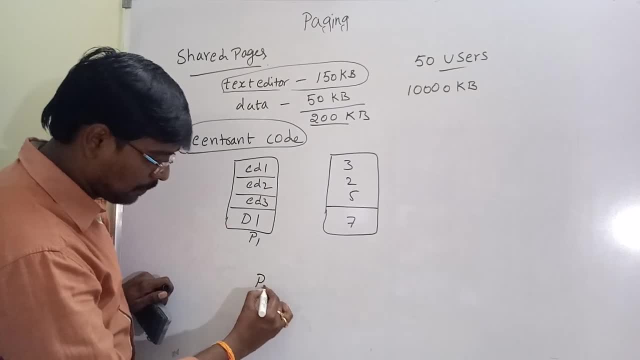 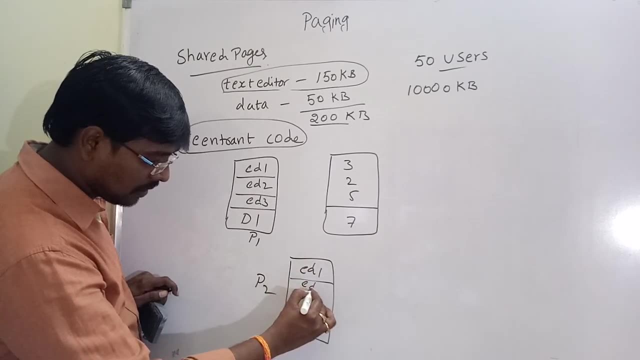 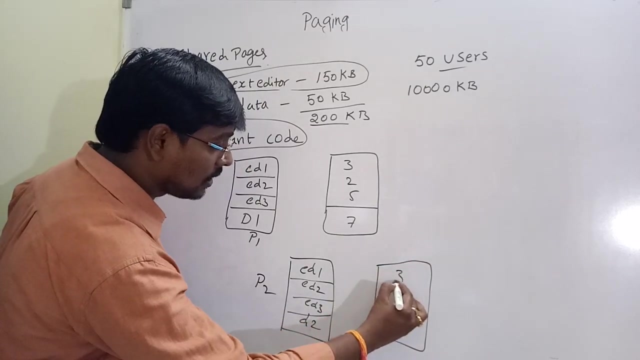 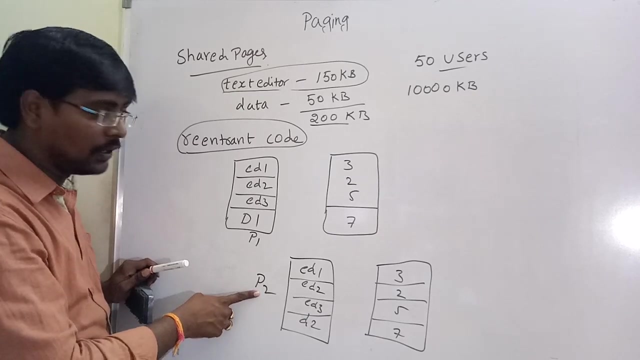 So these are the corresponding frames: Suppose page 2, page process P2.. It also contains ED1, ED2, ED3.. Suppose D2.. Its page table is 3,, 2,, 5, 7.. See this one Here, these two process: P1 and P2, ED1, frame number is 3, frame number is 2, frame number is 5.. 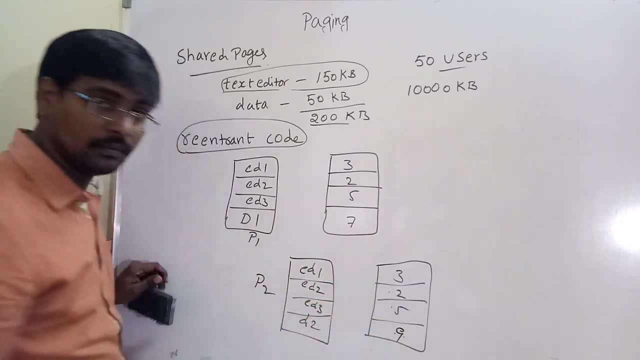 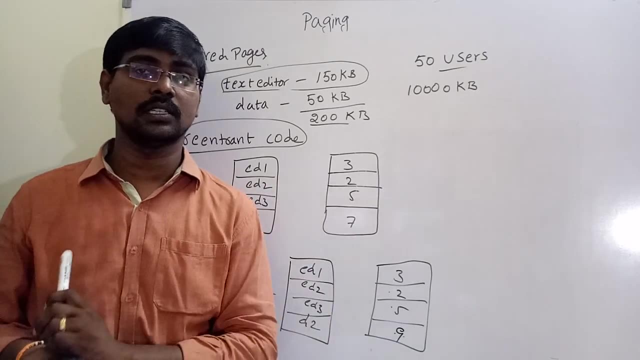 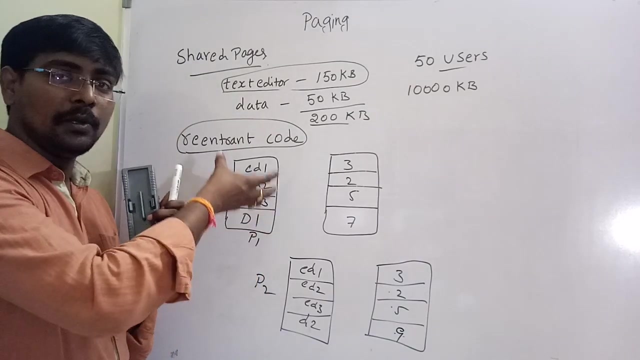 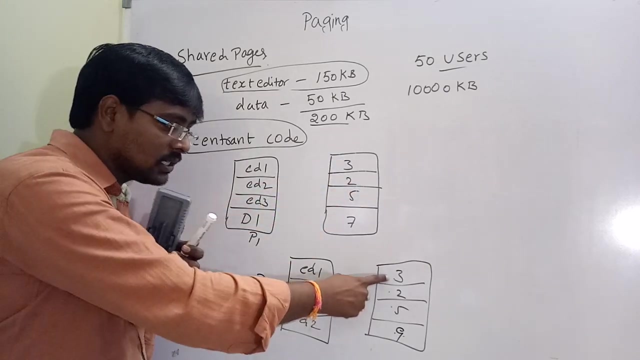 Here also 3,, 2,, 5.. That is, all these two process share the same frames. Share the same frames. This is the concept of sharing. Suppose, if more than one process So want to use the same location, No need to make a different copy, Simply make one copy. Make one copy, All the process, access that particular frame. 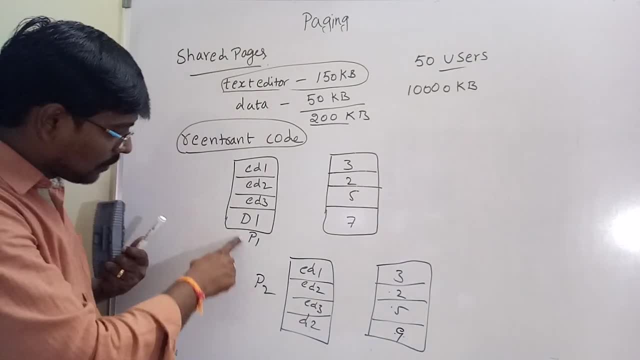 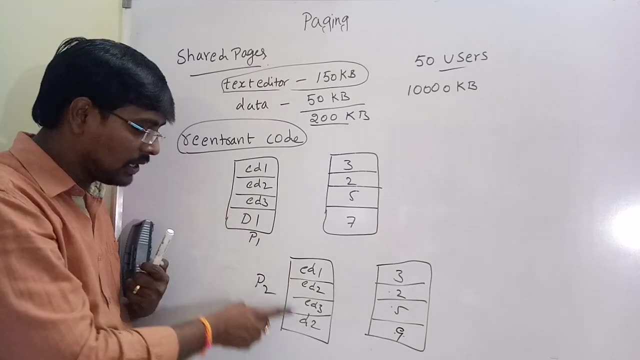 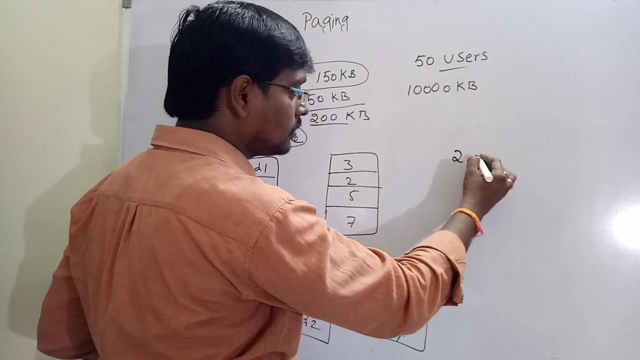 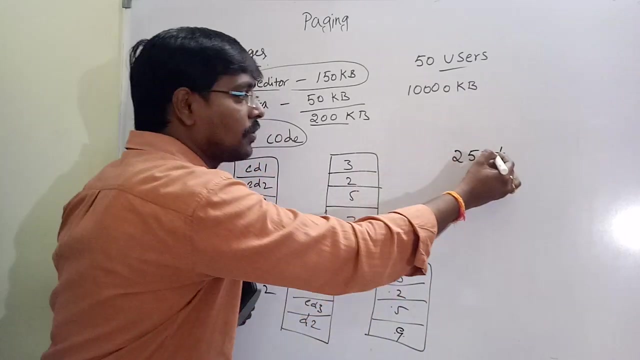 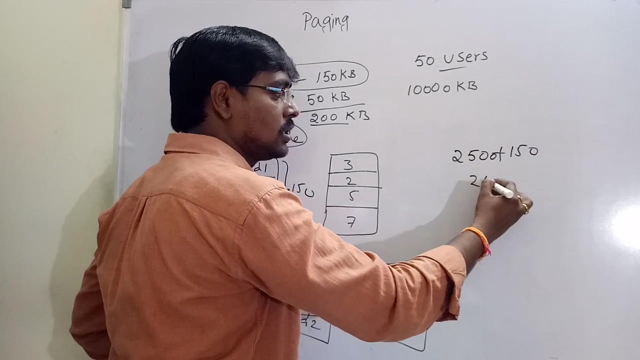 Then how much amount of memory is saved. Suppose some 50 users, All 50 users have a separate data space, only Separate data space only. Suppose data space is 50 KB, So 50 into 50.. 250 KB Plus 250 KB, Sorry, 2500.. 2500 KB Plus this size is some 150.. Plus 150.. That is 2650.. 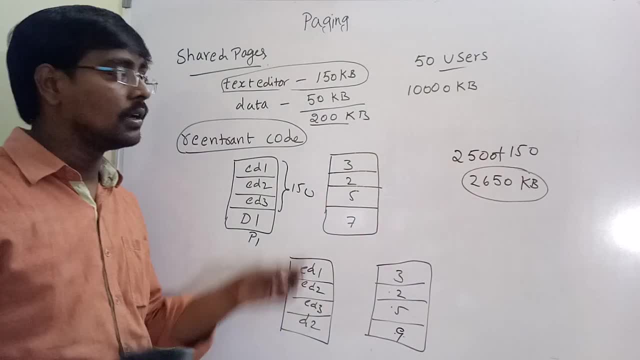 KB is only needed because of sharing, That is, to save the memory. This is the concept of sharing.